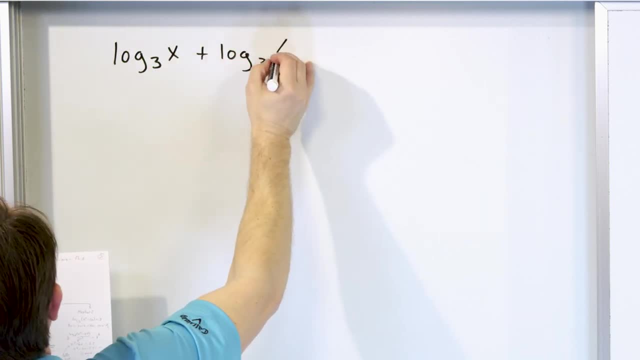 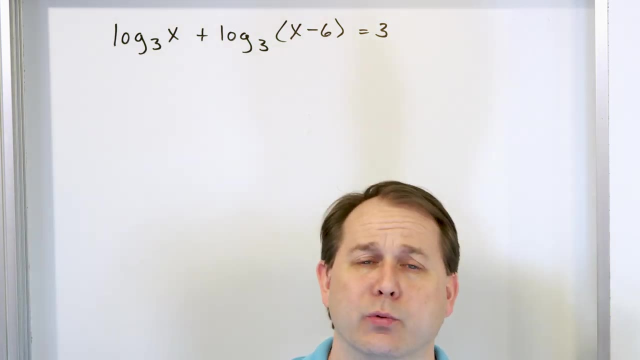 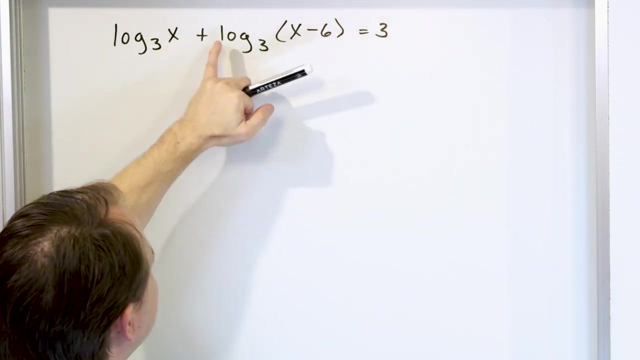 number x plus logarithm base three of some number, x minus six is equal to three. Now this is what we call a logarithmic equation. It has an equal sign, so it's an equation and it contains logarithms. Now, in this case, the unknown quantity is x, but that x appears in two locations. 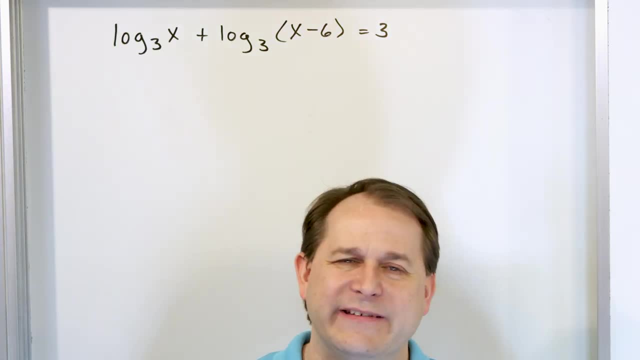 So what we have to do for these kinds of equations is very similar to regular equations. We want to isolate and get x on one side of the equal sign all by itself. That's all we want to do, And we're going to have to use the laws of logarithms to do that. So we see immediately we have a term over. 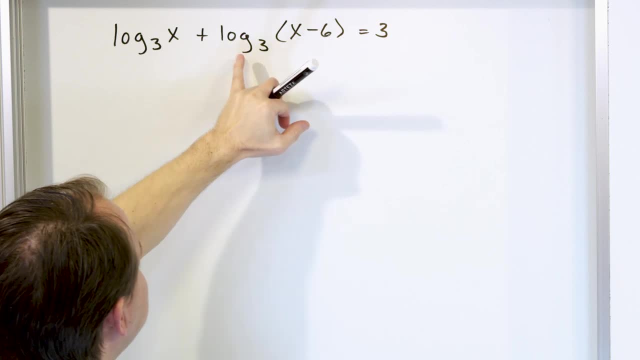 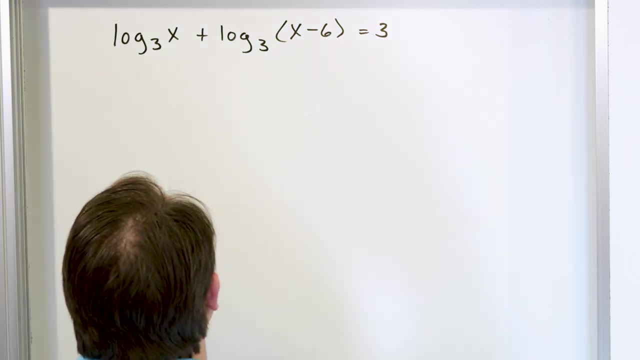 here that's a logarithmic term and a term over here. It's the same exact base And we know that when we add logarithms together we can combine them to basically one single term, as follows. You can combine it like this: It has to be a logarithm. 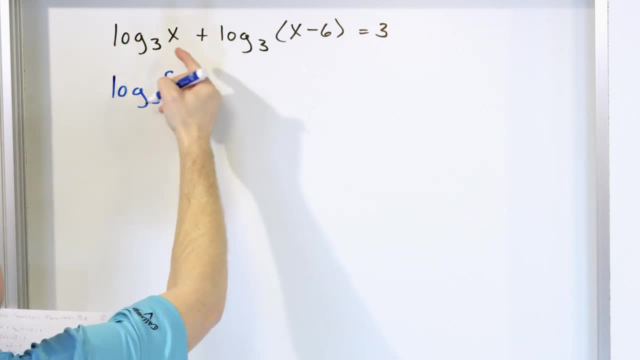 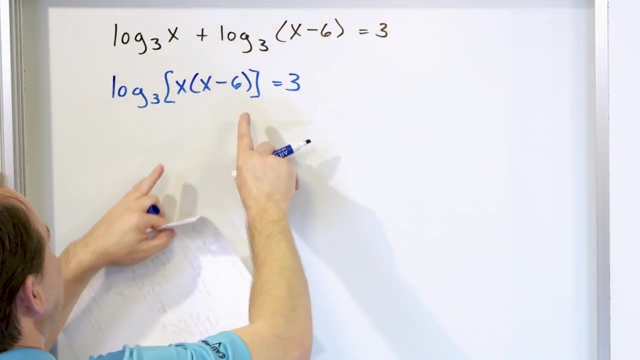 Base three of x, which is this term, times x minus six, which is this term, And that's going to be equal to three. If you do not understand this step, then it just means you never watched the lessons on the laws of logarithms. You can think of it going backwards. We have things. 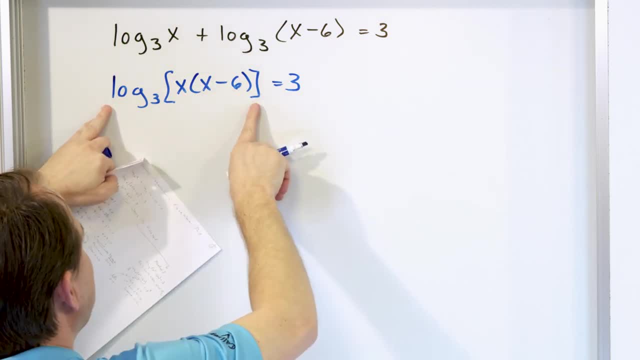 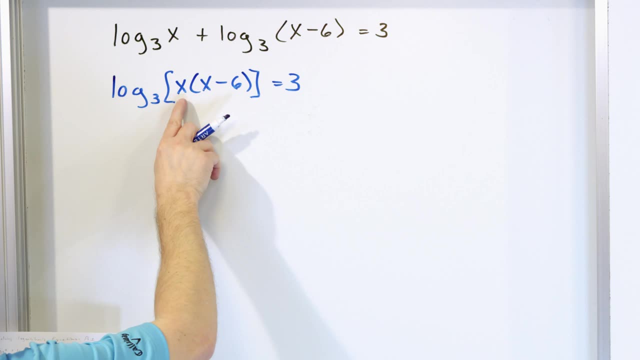 multiplied two things. multiplied this term, times this term inside of a logarithm so we can break it out into addition of those logarithmic terms. That is a law of logarithms we've already learned in the past, So now we have to continue to multiply. 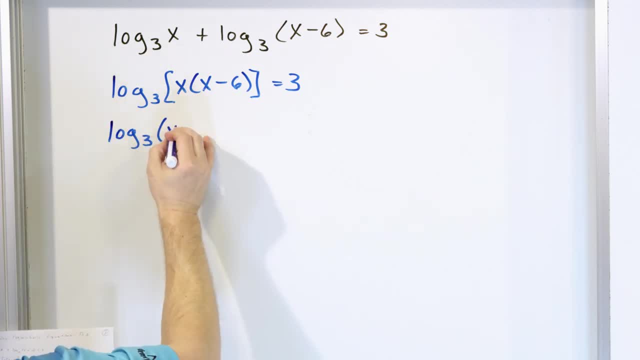 We have to multiply through to get x by itself. Log base three. This is going to be x squared minus six x on the inside, just multiplying the x through, And then we get equal to three. All right, So, as often happens in math, there's almost always multiple ways to proceed When you 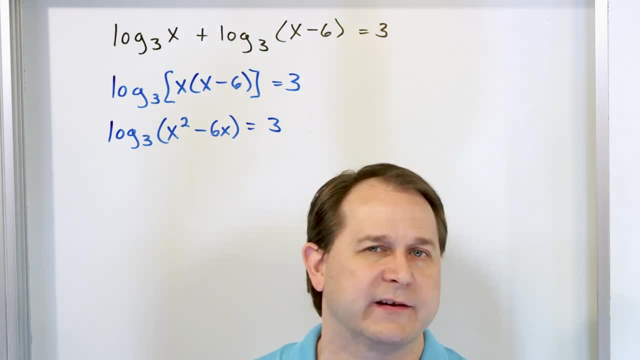 solve equations, there's lots of different paths you can take. So when you get to logarithms, there's actually even more paths you can take and they all should get to the same answer. So if I'm doing something here and you're thinking, oh, I'd rather do it a different way. 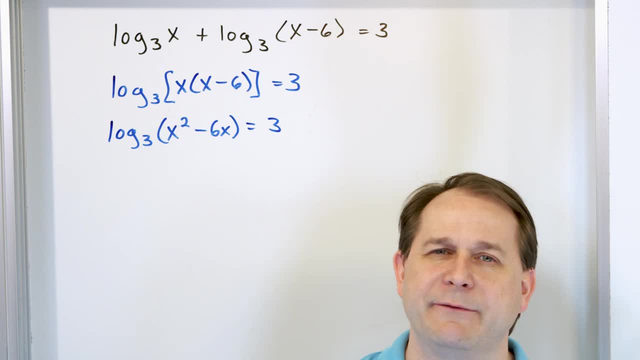 do it your way. As long as you get to the same answer, I'm fine. Now, in some of these problems, I'm going to go ahead and work the problem two completely different ways, because I want you to understand that, no matter what you pick, as long as you're following the correct rules, you're. 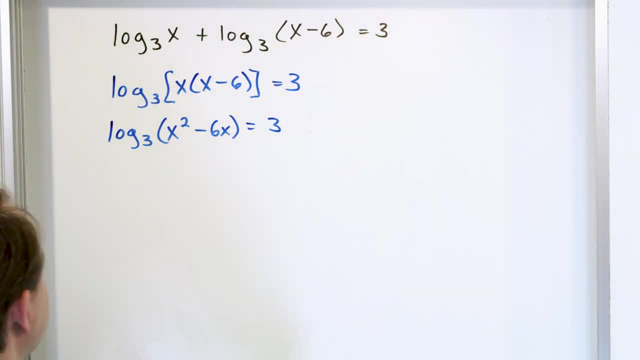 always going to get to the same exact, correct answer. All right, So there's two ways to proceed. I'm going to call this first one method. It's not really a method, but it's kind of the way. I'm doing it: number one, And then over here I'll do number two. So what do I have? This is a logarithm. 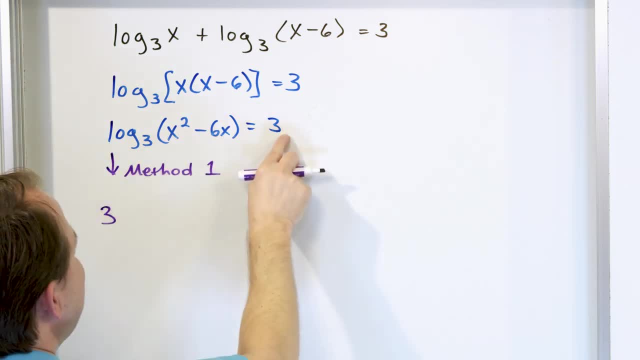 It has a base 3.. So I can write 3,, which is the base, to the power of 3,, which is what's on the right-hand side, is equal to what I'm taking. the logarithm of x squared minus 6x, You see. 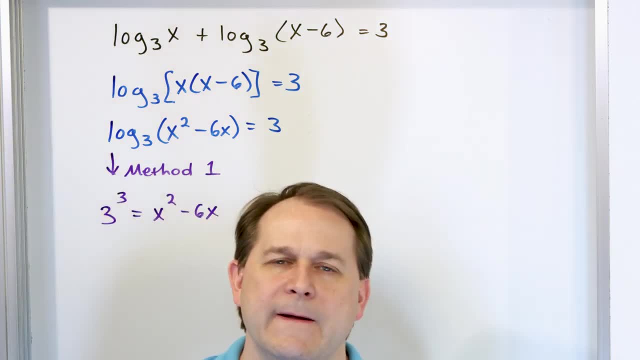 in this way, I've completely eliminated the logarithm from the equation. It's gone, So that logarithm where the variable was wrapped up inside of that logarithm, it's now gone. I don't have to worry about that, because I used the definition of the logarithm, The base, to the power of whatever. 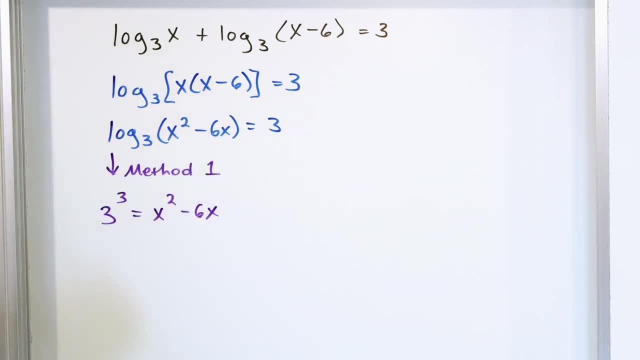 the logarithm returned is equal to this, And that is just simply a polynomial. now. So what you'll have is you have x squared minus 6x- I'm going to move this to the other side- So it'll be a minus sign, And 3 times 3 is 9.. And so what you're going to actually not 3 times 3 is 9.. It's 3,. 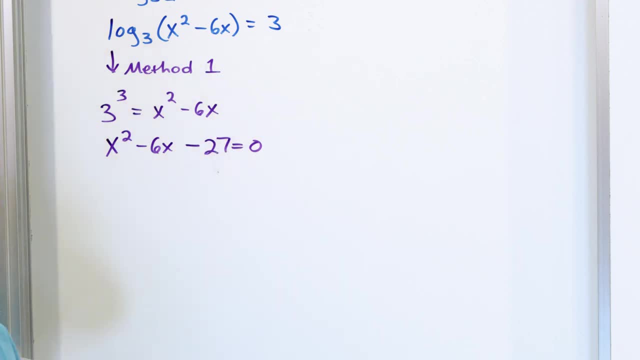 not 3 squared, It's 3 cubed, So you're going to have 27.. Sorry about that. So we subtract it. bring it over here. It's going to be a negative sign: 27. And that's equal to 0.. So now your 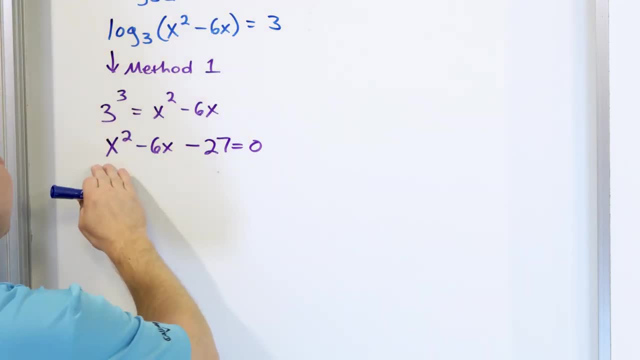 logarithmic equation just now reduced to a polynomial that we've solved many, many times, So let's try to factor this in, Open up parentheses, equal to 0.. x times x. We can pick whatever you want here, but ultimately 9. 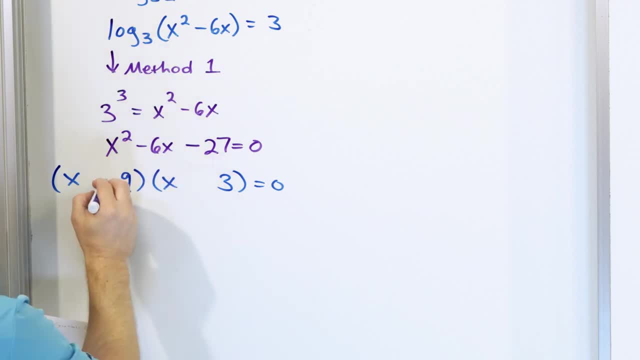 times 3 is going to work. We need a minus sign and we need a minus sign here. So the way that's going to work is minus and plus. Double check yourself: x times x is x squared. This times this is negative 27.. Here's a negative 9x. Here's a positive 3x. You add that, you get a negative 6x. 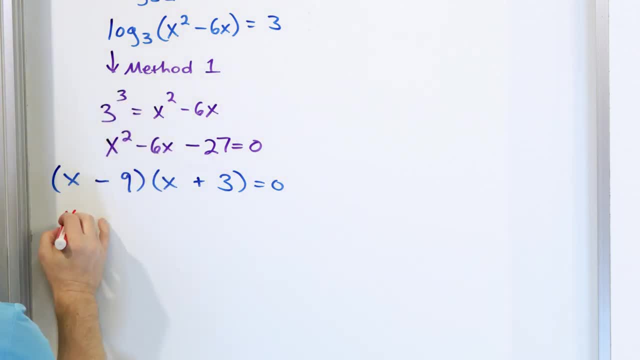 So it appears that we have two solutions. We have x minus 9 is equal to 0. So x can be equal to 9.. And we have x minus 3 is equal to 0. And that means x is equal to 3.. 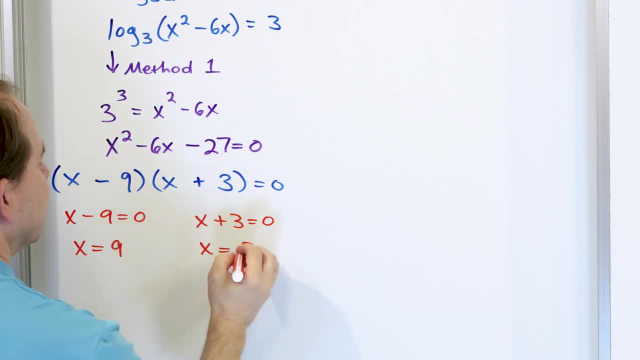 All right. Actually there's a plus sign here, Sorry about that, So this could be a negative right there. So it appears that we have two solutions: x minus 9 is 0.. x plus 3 is 0.. So x can be 9, or x can be negative 3.. So if you were to circle those answers, you would actually 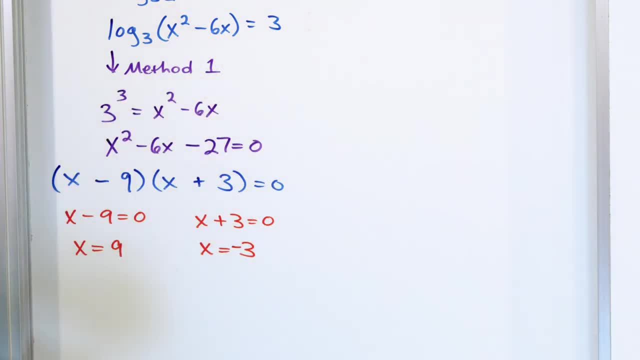 be wrong, or at least partially wrong. Can you spot what the problem is? It's kind of tricky, but the problem is this negative sign here. Right, Remember what you're doing. You're trying to find the values of x that satisfy the original. 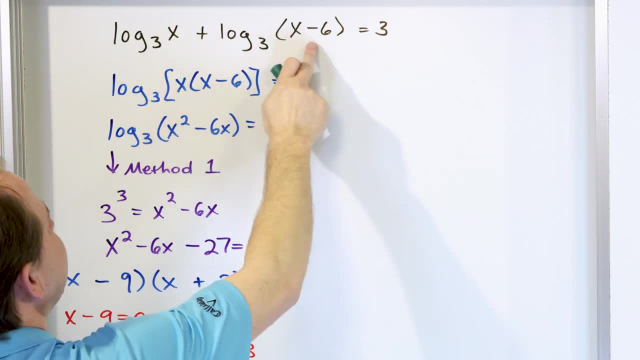 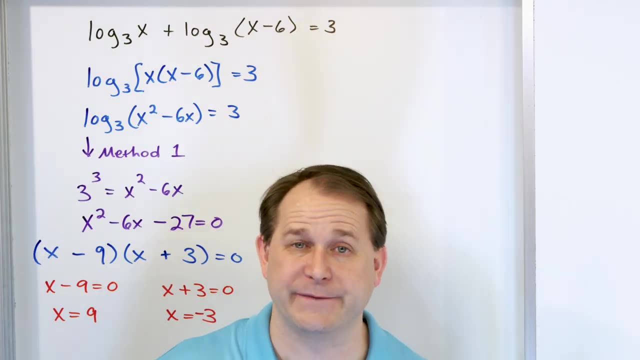 equation that you have, which is this one: x appears here and x appears here, But when you look at the plot of the logarithm function, a logarithm is never, ever ever defined. when you stick a negative value into that logarithm, It doesn't exist, Or at least it doesn't exist in. 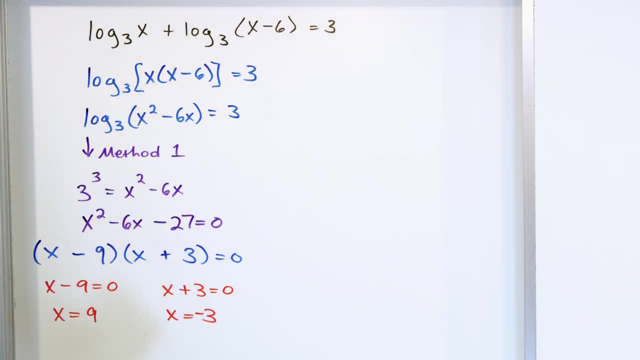 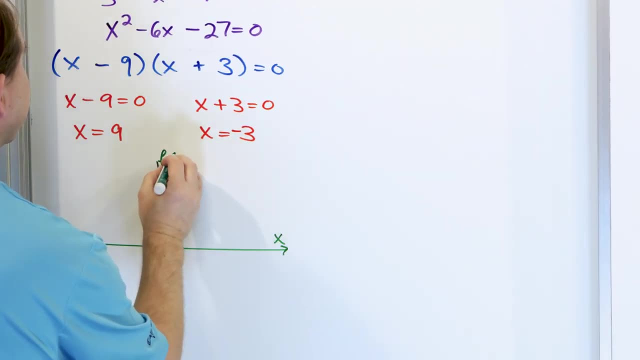 terms of real numbers. Why is that? If you remember back to the plot of a logarithm, it's the inverse function, right? So if this is x and this is f of x and we're plotting a logarithm here, then what's going to basically happen is it goes through the number 1.. That's this spot, right here. 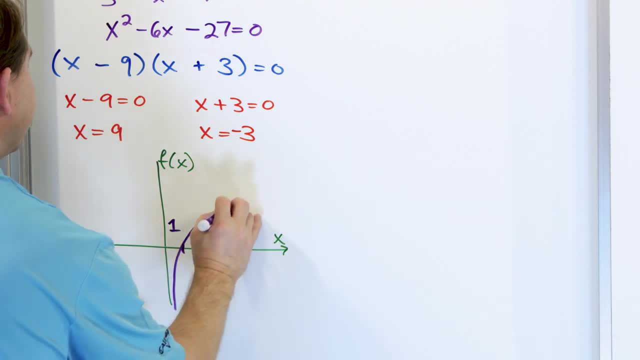 It starts very close to the axis, It goes through this point and then it bends over something like this. So this is an asymptote: It never really gets to the axis right here. So these are negative values of x: negative 1, negative 2, negative 3.. And this is positive 1, positive 2, positive 3,. 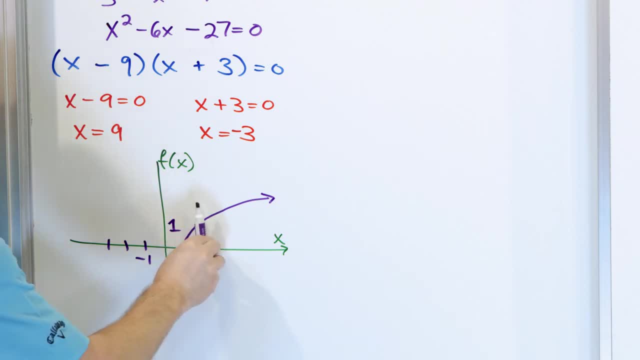 and so on. So the logarithm has values for 1,, 2,, 3,, 4,, 5,, 6,, 7, and also very, very close to 0, like 0.5, 0.3, 0.1, 0.0001.. But it does not exist over here. You cannot put a negative. 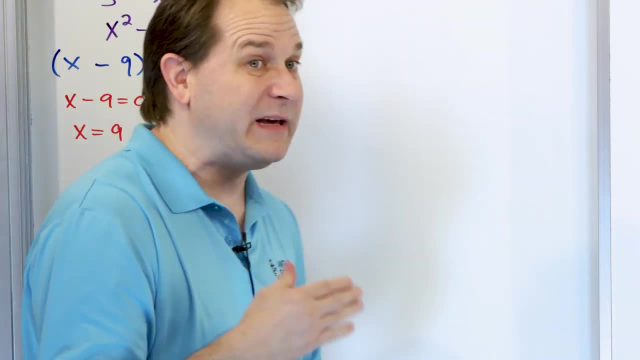 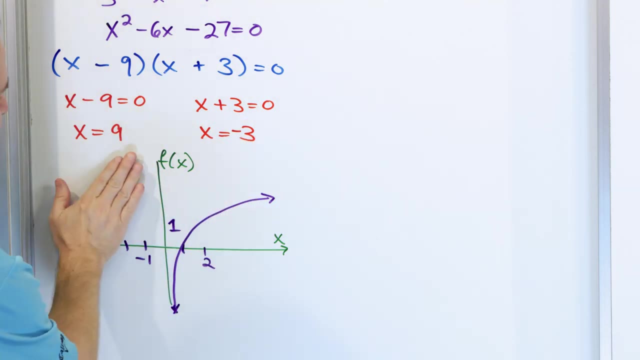 value into a logarithm, And this comes about because this logarithm is a reflection of the exponential function. It's a reflection of an exponential function across this diagonal line. y is equal to x. So if you can imagine an exponential function doing something like this, 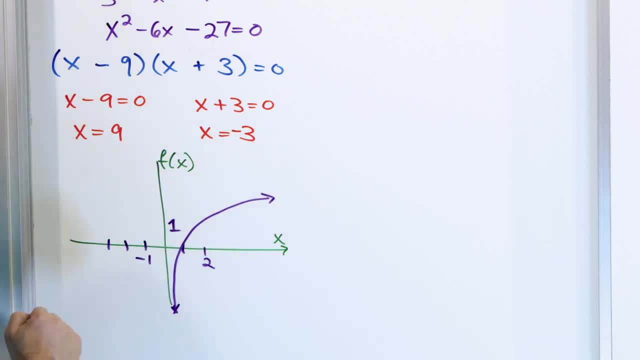 then reflecting it gives the inverse, And that's why it's down here. So, just like an exponential function doesn't exist down here, a logarithmic function does not exist over here, because it's a reflection. So what you need to know is that negative values are not allowed to be stuck into. 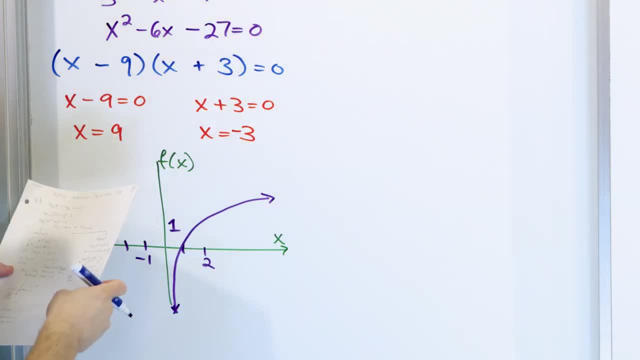 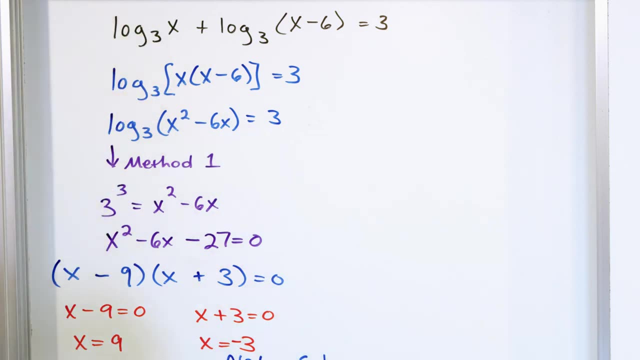 logarithms, And so you cannot have a negative value like this. So what you say is not a solution. If you take a negative 3 and try to stick it in a calculator, it's going to give you an error because it's not defined. 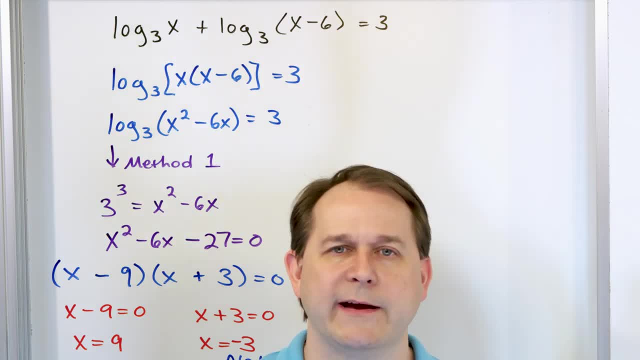 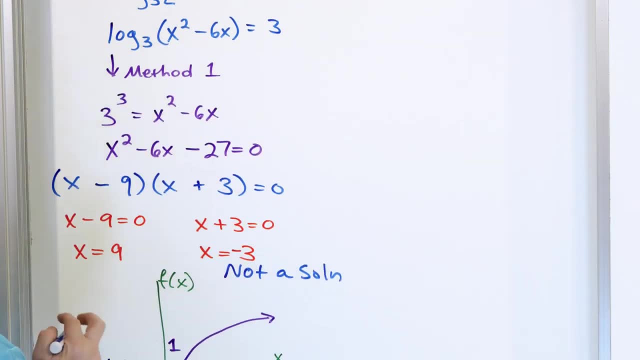 It doesn't exist. It's like saying: give me a square rectangle, square rectangle, I'm sorry, a square triangle. or give me a square circle. It's not going to work. There's no, it's not defined. So we throw away this and we say: this is our solution. We have one solution. 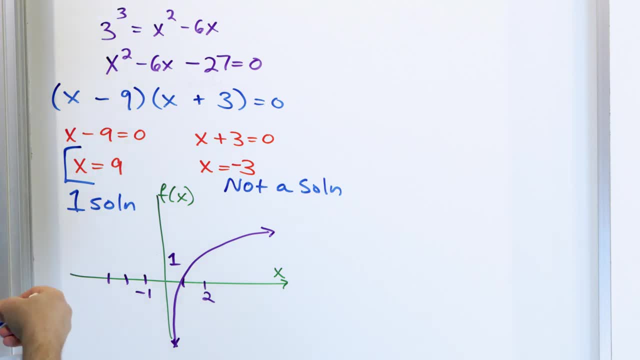 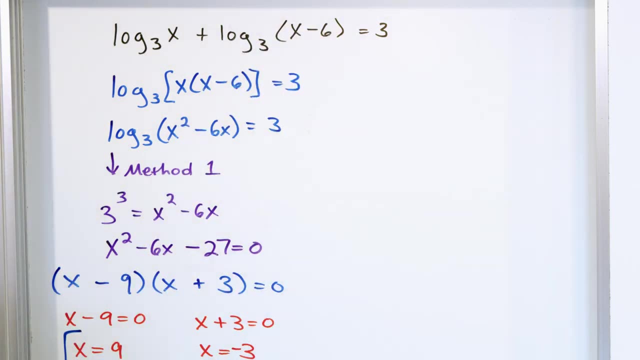 of this equation. All right, One solution of this equation: If you stick the number nine in here and calculate this log and here and subtract and calculate this log and add it, then you're going to get the number three. Now that was method number one, using the definition of the logarithm. 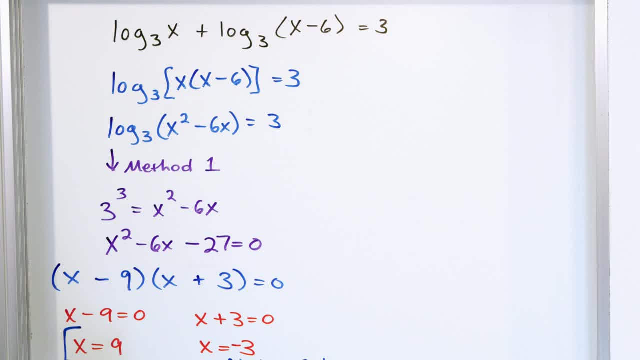 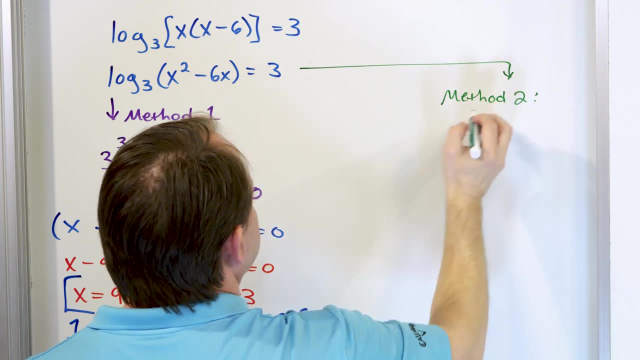 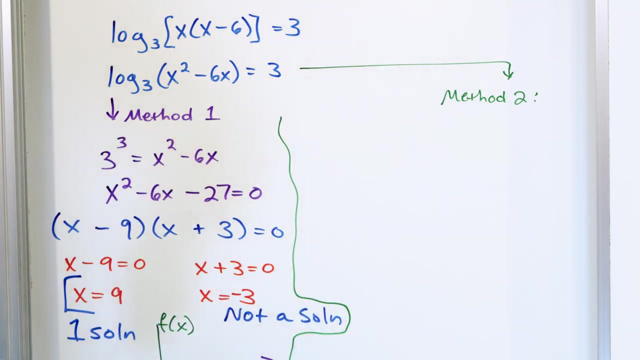 There's always different ways to do a problem, So I want to talk briefly about what I'm going to call method number two, because there's always more than one way to do something. So let's go around here and try to keep things as tidy as I can, Okay? So we have this logarithmic equation here. We 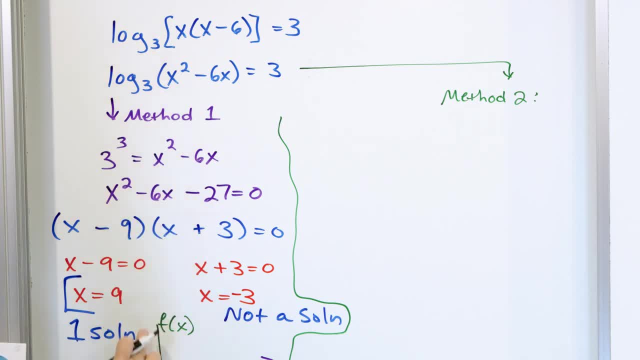 combine the logarithms, We get down to this point. This is the point where we branch off and we say there's two methods. What else can we do at this step, right here? Remember we talked about the fact that a logarithm is not a solution. Remember, we talked about the fact that a logarithm is not a 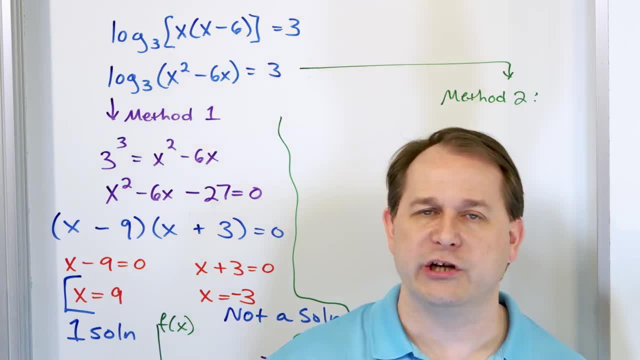 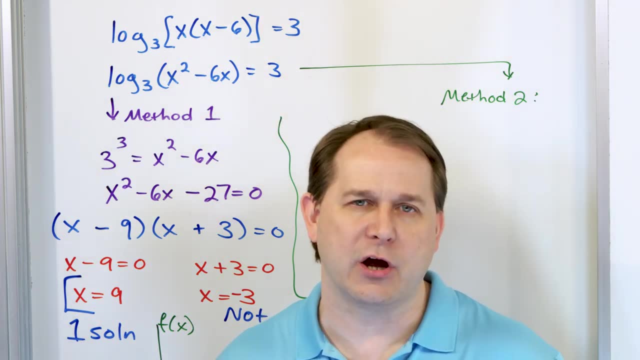 solution. Remember, we talked about the fact that a logarithm is the inverse function of an exponential. They are opposites of one another. They annihilate each other, They kill each other, They undo each other. Whatever word you want to do, the opposite of a logarithm is an exponential. 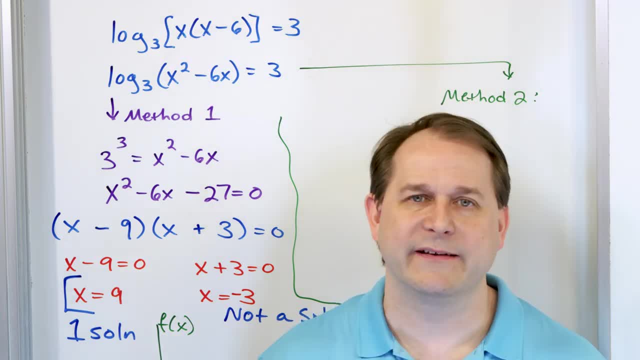 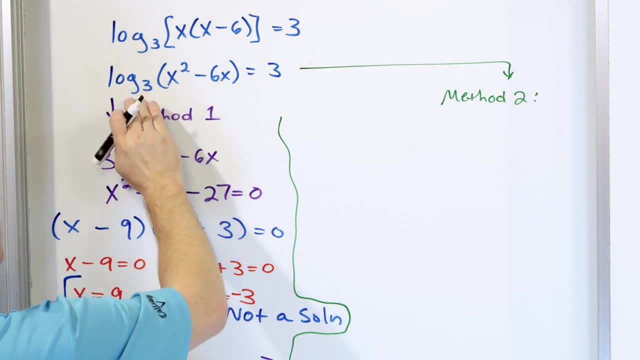 The opposite of an exponential is a logarithm. We've done problems like this in the past, but this is the first time where we're going to solve kind of a more complicated equation using this. So if I don't want to do this, but I want to start at this point, then what I can do is I can. 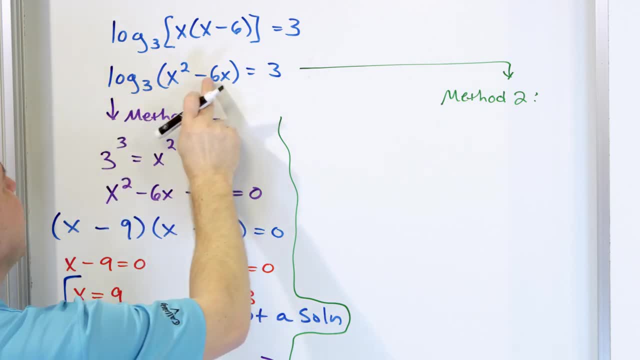 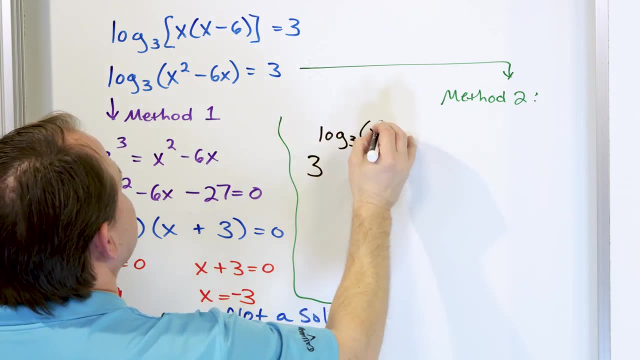 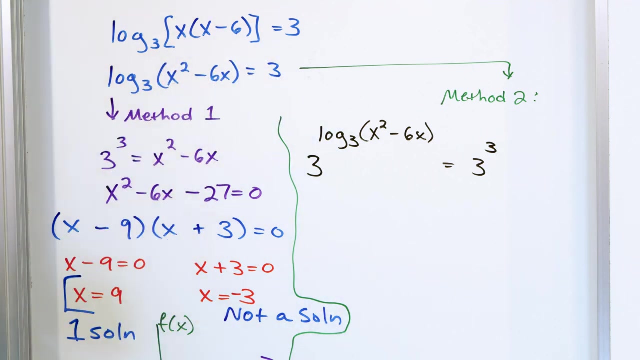 since this is a logarithm that I want to get rid of, I can raise, both sides, A base of three. I can say three to the power of logarithm base. three x squared minus six x is equal to three to the power of three. See what I've done. I can do anything I want to both sides. 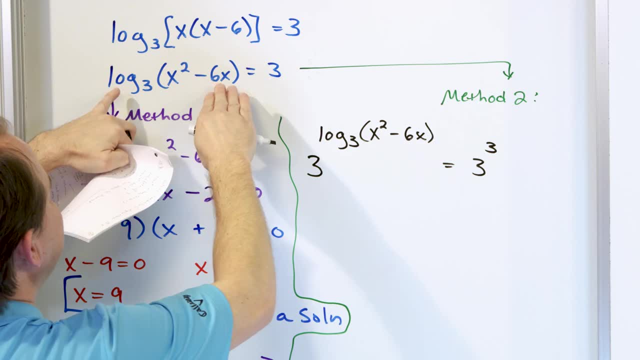 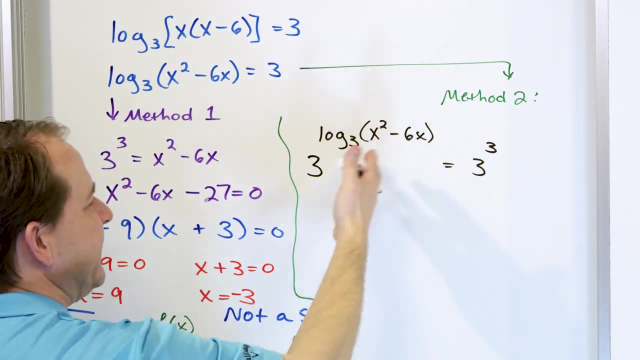 of this equation As long as I'm doing it to both sides. I choose to raise the left hand and put it in the exponent of a three, and the right hand side I'm going to also put it in the exponent of a three. So I'm basically the equation is still balanced. I've raised both sides. 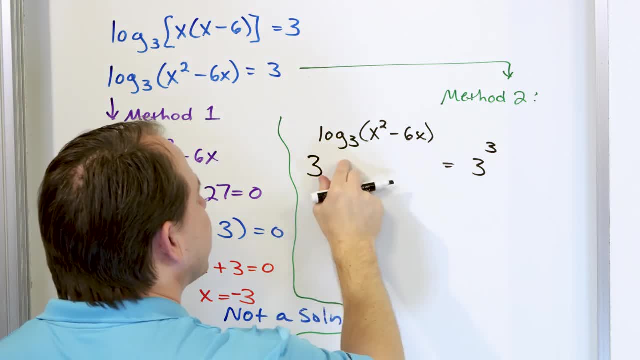 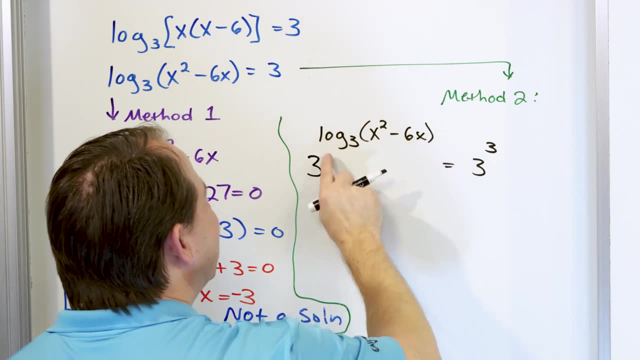 to the power of three. but here I have a power of base three. Then in the exponent I have a logarithm base three. So the exponential base three cancels or annihilates or kills the logarithm base three. And all I have left down here is x squared minus six x. 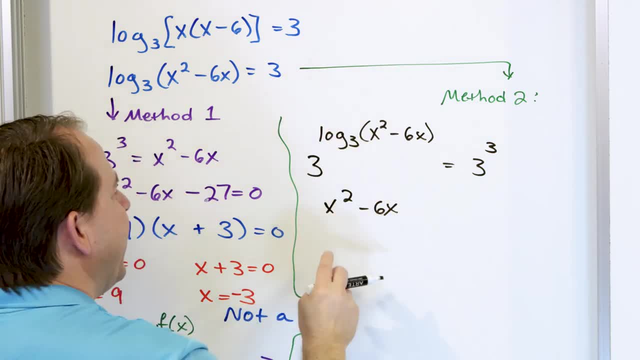 poof This. it's like you could draw a line through the log and through the base, And this is what I have left. equals not nine. I keep wanting to say nine. This is three. cubed is 27.. Look at what I've. 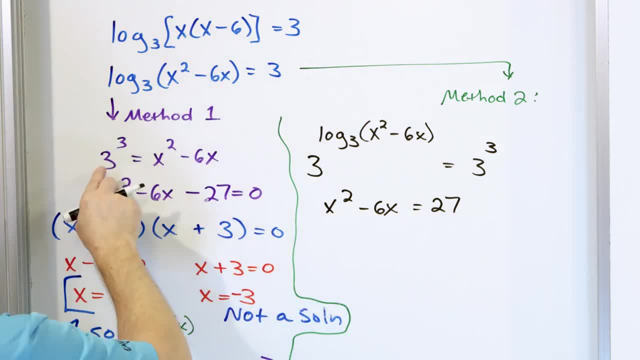 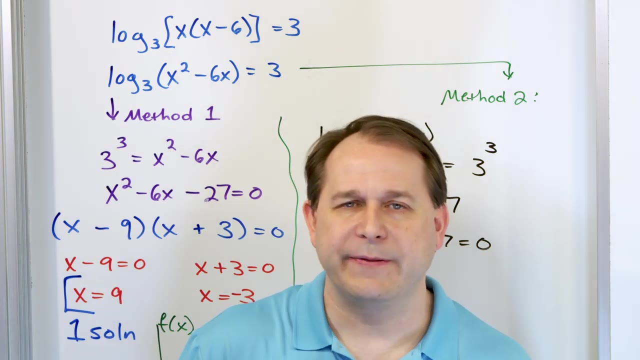 written down here: X squared minus six x is equal to 27,, which is exactly what I have here. X squared is equal to zero. It's exactly the same polynomial we wrote down right here. So, whatever way you want to do, I want you to do that. However, I do want you to start thinking. 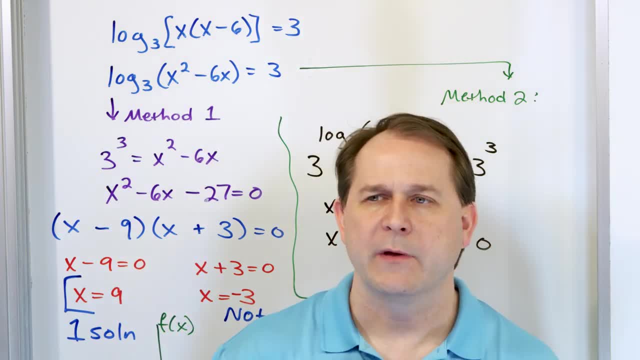 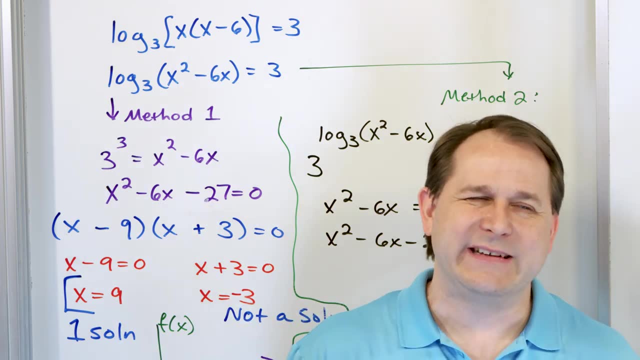 about: oh, I want to kill that logarithm. I'm going to raise that thing to an exponential. Oh, I want to kill that exponential. I'm going to, I'm going to take a logarithm on that boy because then I can get rid of it. Right, I know that it doesn't really seem like it's. 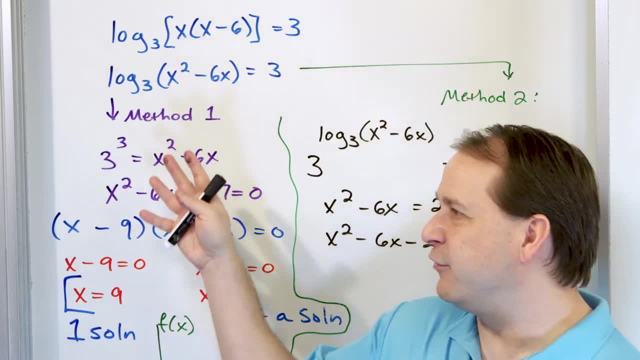 something you want to do in these kinds of problems. here It seems like maybe it's easier to do it this way and whatever you want to do, But I'm telling you that as you get to more complicated problems, you're going to get more complicated problems. You're going to get more. 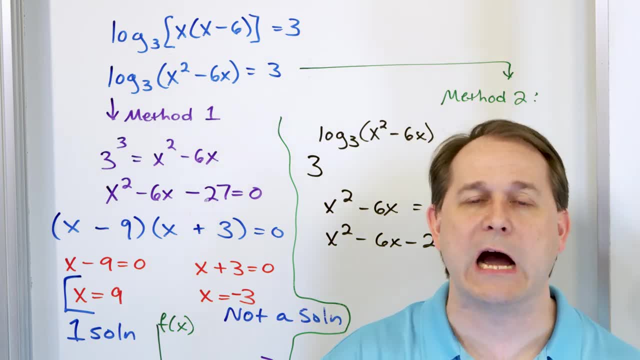 complicated problems. You're going to want to annihilate and eliminate both sides of an equation by doing the opposite or the inverse operation. And that means if you have a log, then you take the exponential of both sides to kill that log, and so on, And you get exactly the. 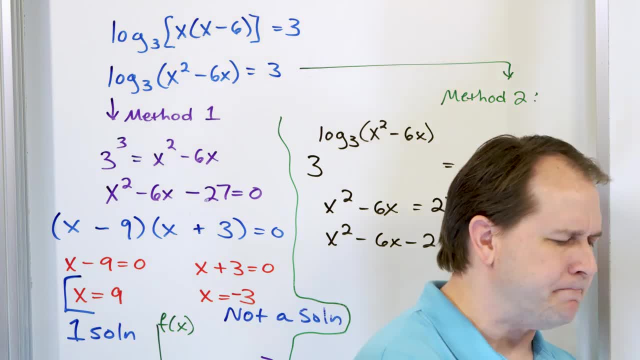 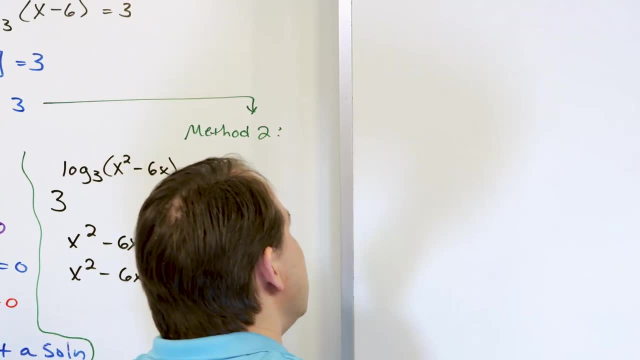 same solution either way. We're not going to do that every single time. I'm not going to solve the problem twice every single time, but a few times along the way I will do that. Problem number two: Let's say we have logarithm, and here's something weird: The base is actually not a number. 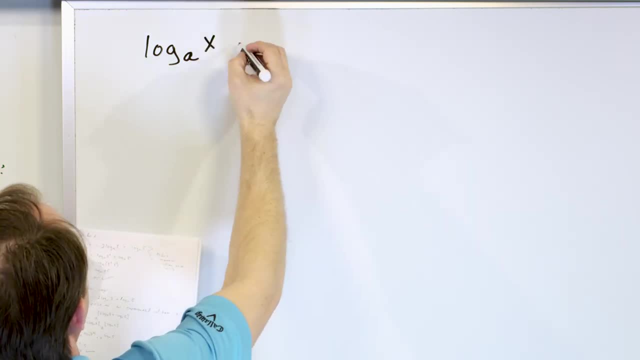 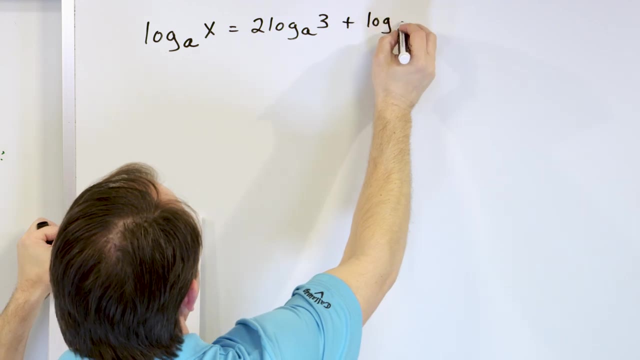 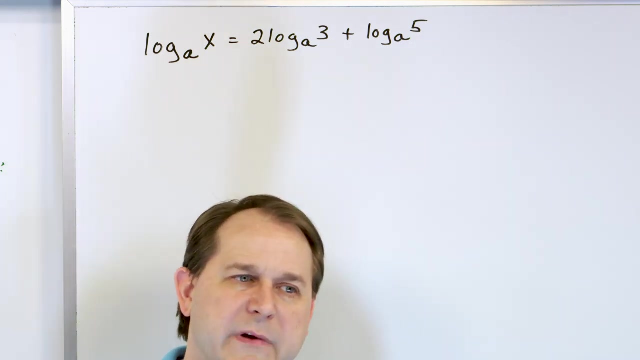 Let's call it a. I'll explain in a second. Of the variable x is equal to two times a logarithm base a of three plus logarithm base a of five. All right, So you might look at that and say: I've never seen an equation like that. It makes no sense at all. Well, it's because you haven't. 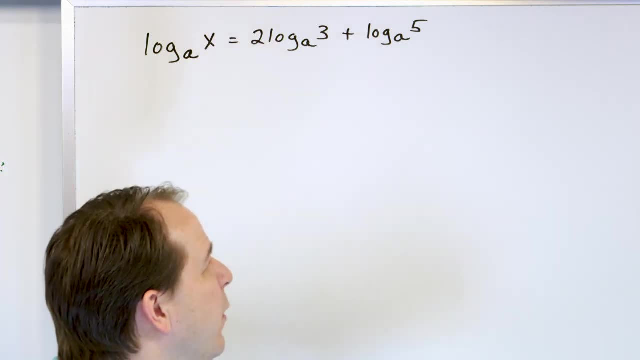 seen it before. So once you see it the first time, it's not so scary. What's going on here is, you know, normally we have bases of logarithms: base two, logarithm base three, logarithm base 10, logarithm whatever. Here I'm just saying. 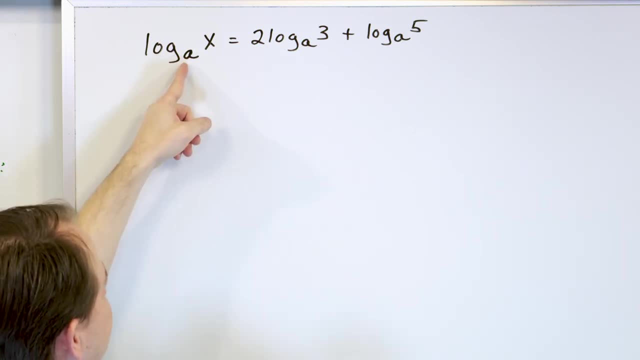 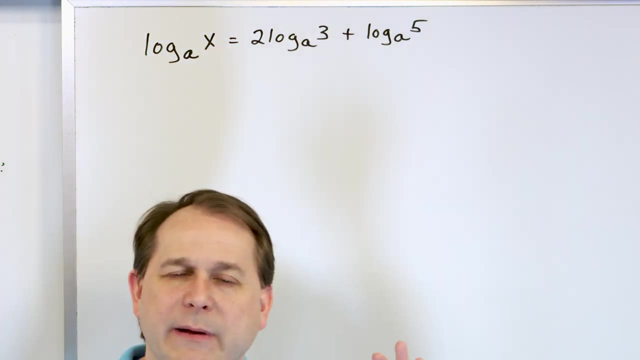 I don't care what the base is. It's base a. Some number is here, I don't know what it is, but it's something, And whatever that is, it's the same base for this logarithm, and it's the same base for this logarithm. A is not what I'm trying to solve, for though I'm trying to solve. 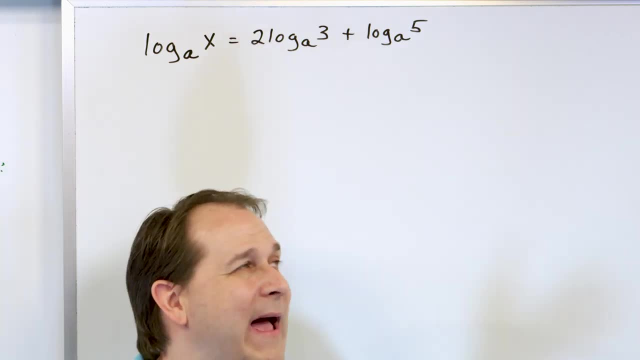 for the variable x. X is my unknown. It just so happens that in this equation, base a base, a base a doesn't actually matter. You're going to find out, as we do, the solution that the base, the particular base of this logarithm, it doesn't matter if I have a base two in all three of those. 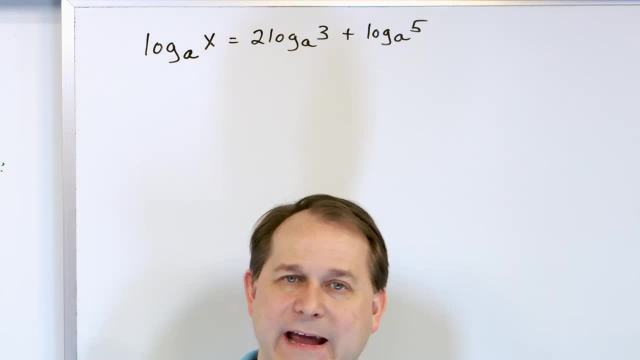 locations, or a base 10. in all three of those locations, the n-th is going to be the base of a answer will be the same, So don't let that stress you out. Just treat it as a base and follow the rules of logarithms. What do I want to do? Again, there's a couple of different ways I'm going to. 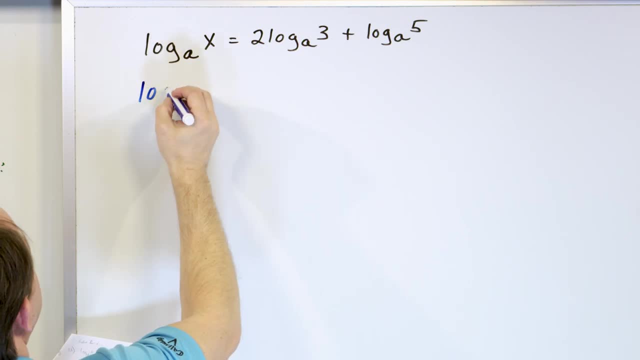 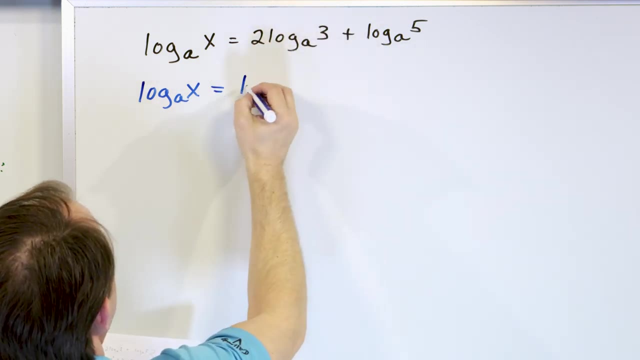 do this. but let's start working on the right hand side. Let's say on the left, log a of the unknown variable x. Here I have a two times log, so I'm going to bring that two and put it in the exponent. That's one of the rules of logarithms that we learned in the past, that I can take an. 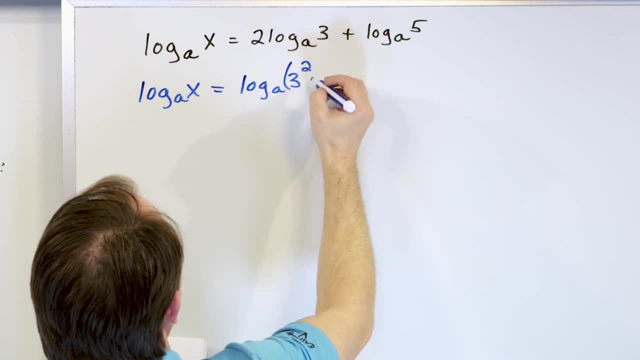 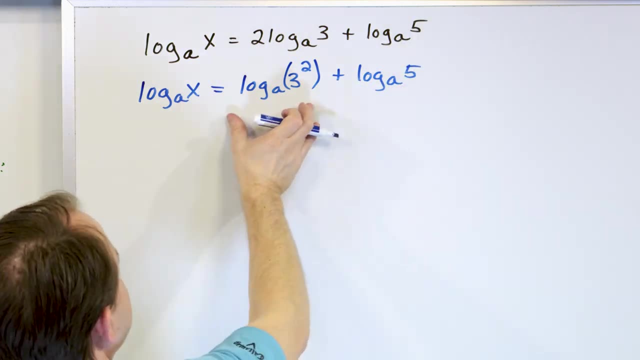 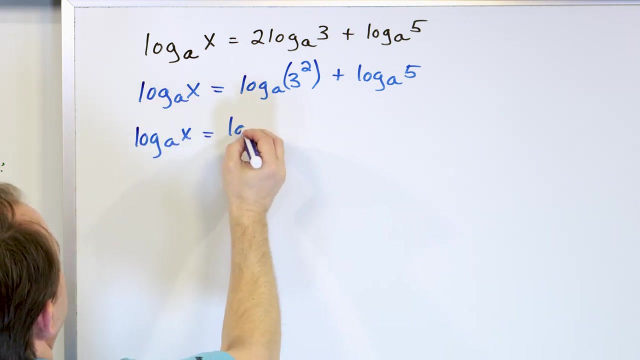 outside multiplier number and move it into the exponent on the inside of a logarithm like this, And then I have log again, base a of the number five. So on the right hand side I have a logarithm plus a logarithm and I can now combine those Logarithm, base a of the number x logarithm. 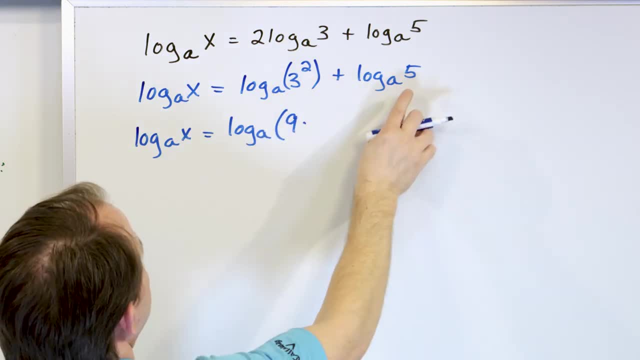 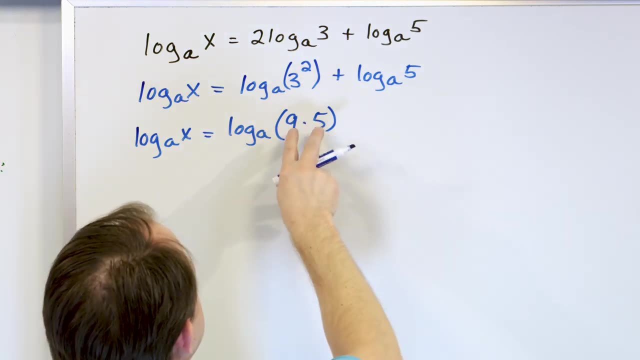 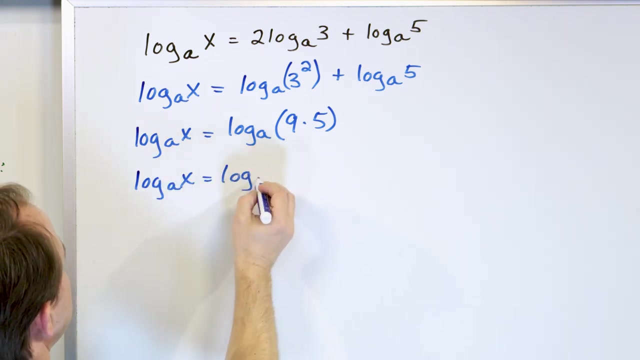 base a of three times three is nine times the five. So I'm basically multiplying inside, because multiplying on the inside of a logarithm becomes addition of logarithms. So when I continue, I have log base a of 45. And now you. 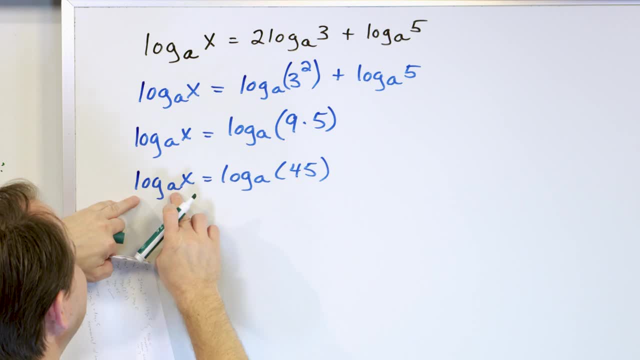 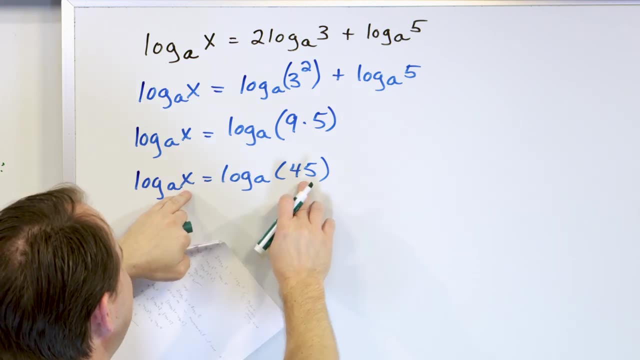 see exactly what the solution of the equation is. I have a base- a logarithm- on the left and a base- a logarithm- on the right. It's the same exact logarithm, same exact base. So the only difference between the two is what x is, and it has to be equal to 45.. And that's how you write the answer. 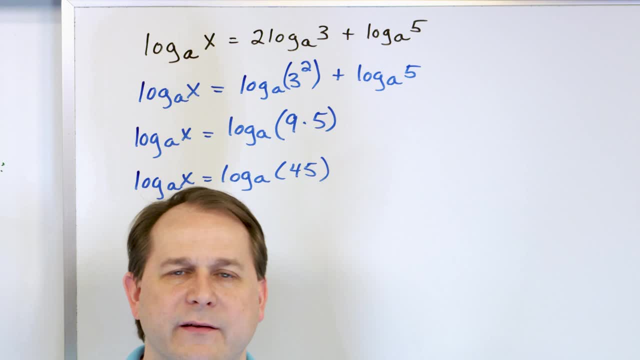 I got it into a position where everything else was the same, so that x had to be equal to what x had to be equal to 45. And now you can see that it doesn't matter what base you put in here. If I chose this to be base two, base two and base two, all that would happen is I would get. 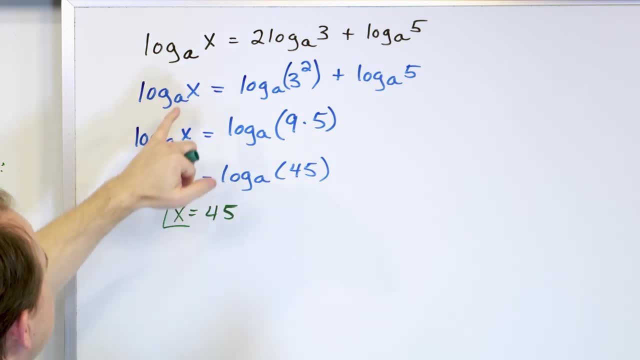 base two here and base two here, x would still be 45.. If I choose a base 10, 10, and 10,, all that's going to happen is this will be base 10 and base 10.. x will still be equal to 45. 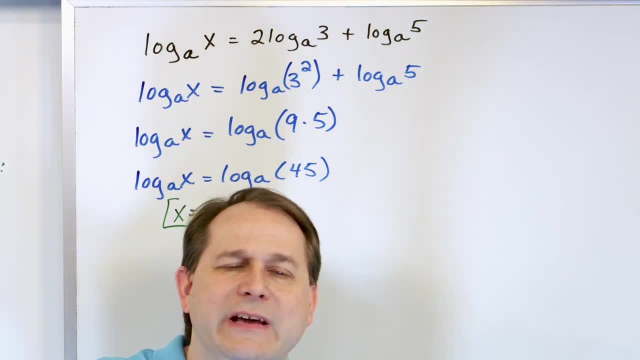 Don't get so wrapped up when you see that you don't think you can get to the end from the beginning. You have to just start working and start carrying things through logically. Okay, Now, there's always one more than one way to do something, and I want to show you that way. 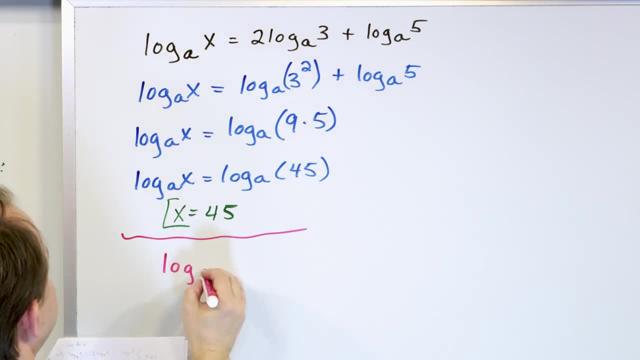 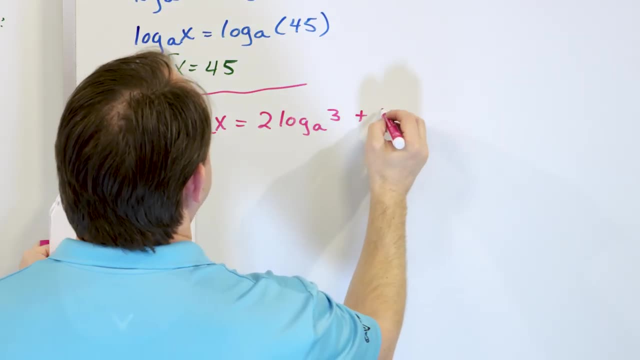 Let's write the equation over again: Log base 0 of x, 2 times log base a of 3, plus log base a of 5.. All right, So I told you. I said you know, ultimately I want this. 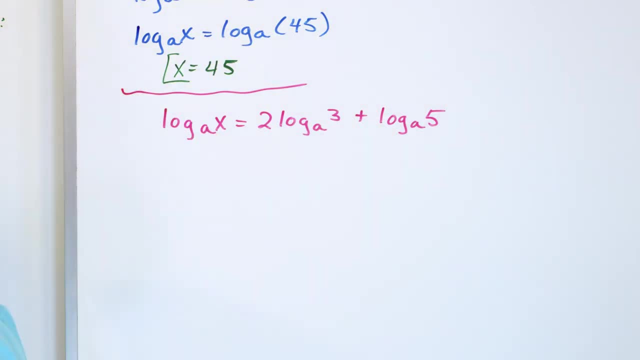 x variable over here. so forget about the rest of this thing. I want x by itself, But x is wrapped up inside of a logarithm. a base, a logarithm. How do I get x by itself? It's wrapped up inside of. 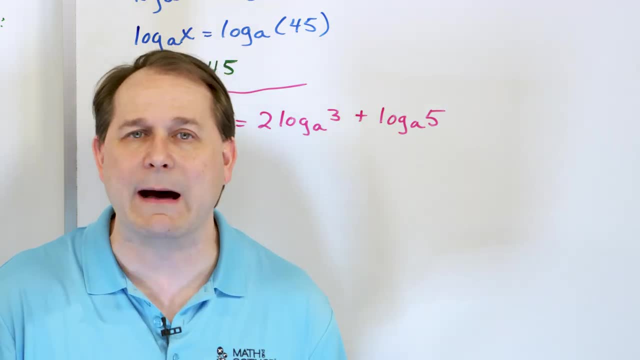 a package. How do I get rid of that logarithm? Well, I have to do the inverse. the opposite function, The opposite of a logarithm, is an exponential function. So if I take the left-hand side and I say base a, and I raise it and put this thing in the exponent base a of x, I have. 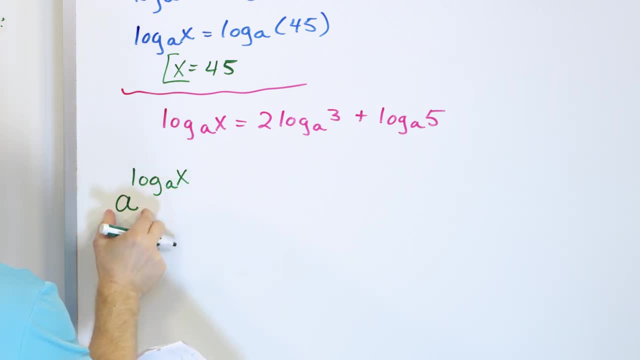 taken what I have and I've raised it to the exponential of the base- a exponential, So I have an exponential and a logarithm up here. They cancel each other. So that's how x is going to drop out on the left, but I have to do the same operation on the right-hand side, So it'd be a 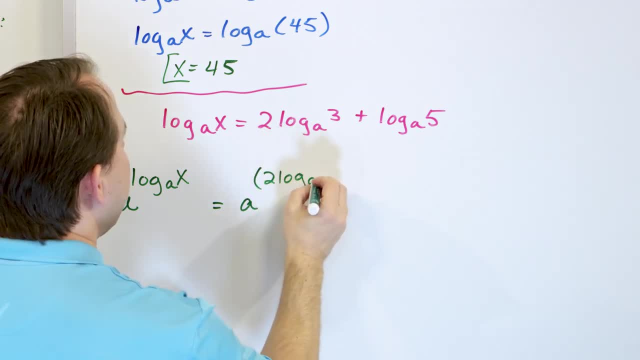 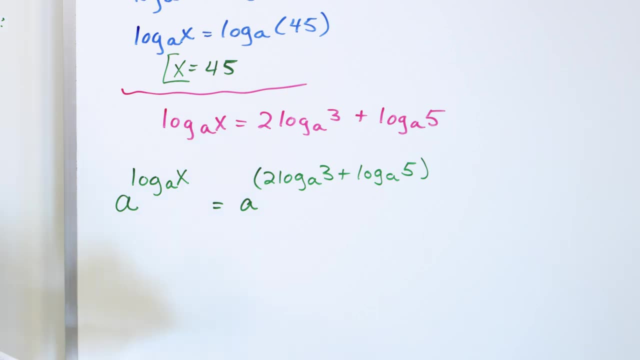 to the power of two times. log a three plus log a base a five. I know it looks crazy. All I'm doing is I'm raising the left-hand side of the equation to the power a, to the power of that and then a. 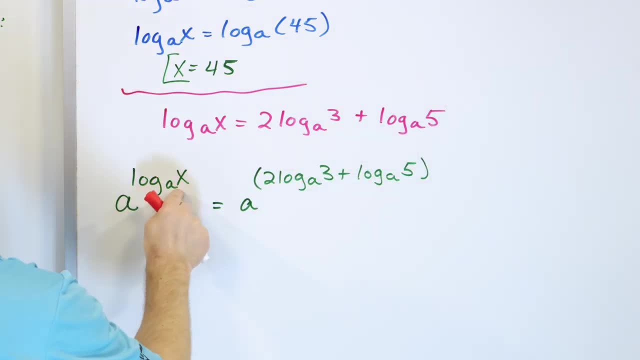 to the power of this. But the nice thing about it is because log is exactly the inverse of a, then on the left-hand side the only thing left is x. It drops out. It's like it cancels with it. Just like four over four, they cancel. Five over five, they cancel. Ten over ten, they cancel. 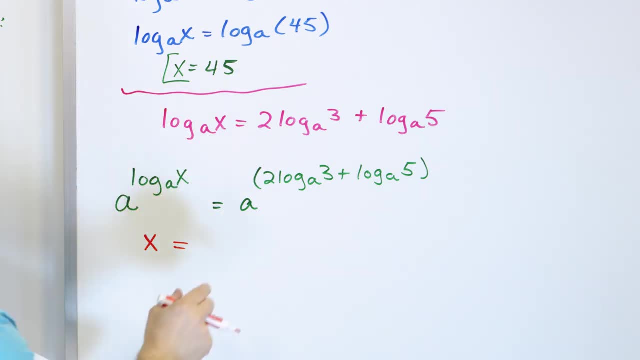 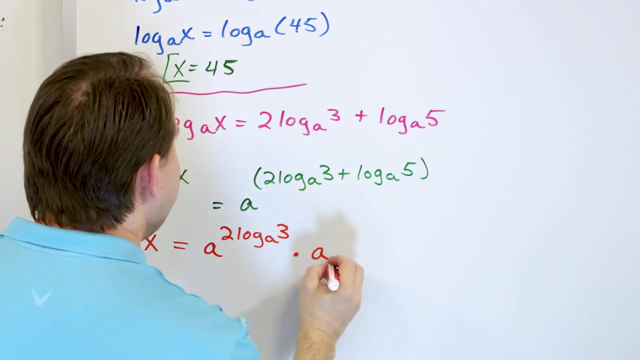 a to the power of log a. they cancel, So the x drops out. On the right-hand side I have all of this stuff, But notice that in the exponent here I have a plus sign, So I can write this exponent as: a to the power of two log base a three multiplied by a log. 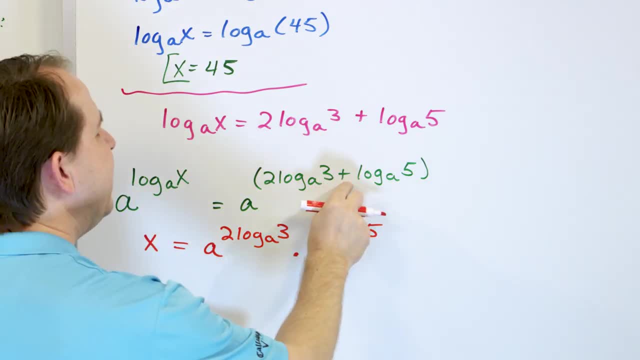 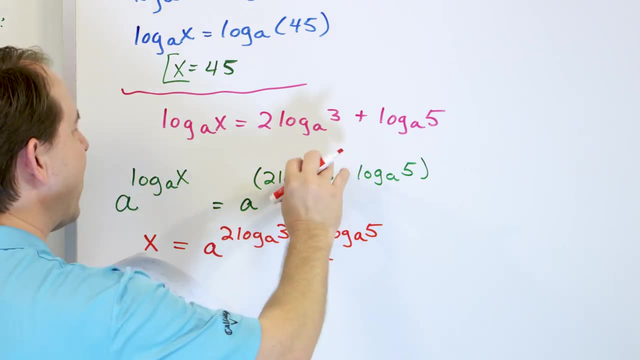 base, a five. How can I write it as a multiplication? Because these exponents are added. So, because the base is the same, I can add these exponents, which is exactly what I would have here. So I'm just breaking it up going in reverse. I have an addition of exponents, so I'm going to treat it. 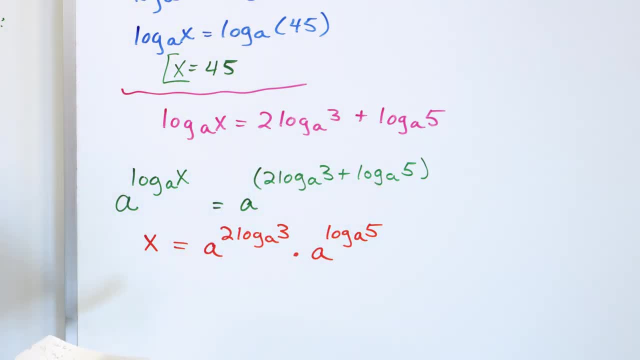 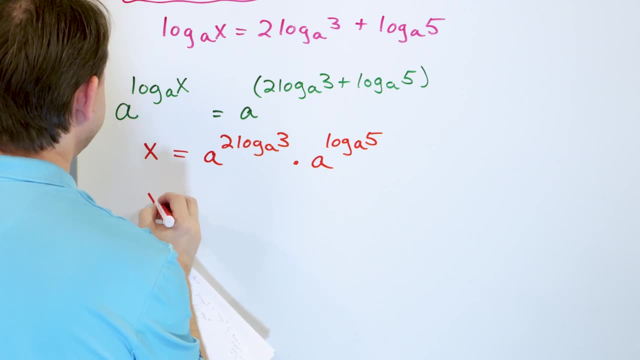 as multiplication And I can add these exponents and get what I have there. So now notice what's going on Over here. I have two times log base a of this, So I need to take care of that. So it'll be a log base a three squared. 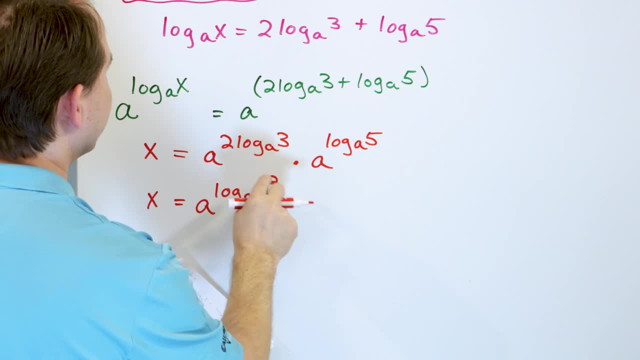 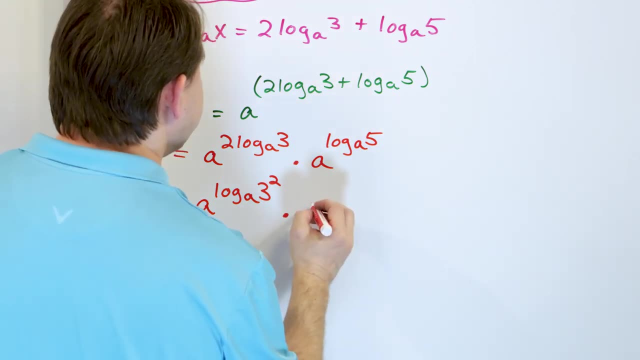 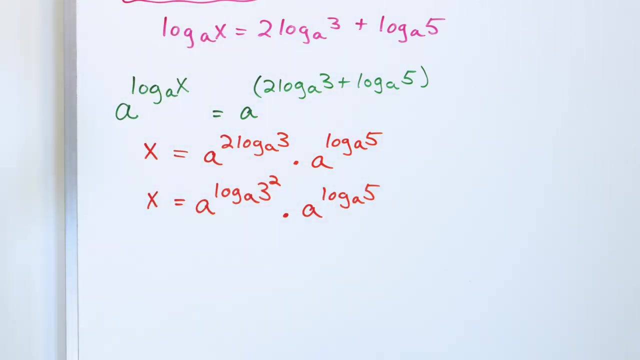 This floats in front and goes into the square here because it's sitting outside of a logarithm. That's another one of our rules of logarithms dealing with exponents Multiplied by a raised to the power of log a to the fifth, Not to the fifth log of the number five. So here: 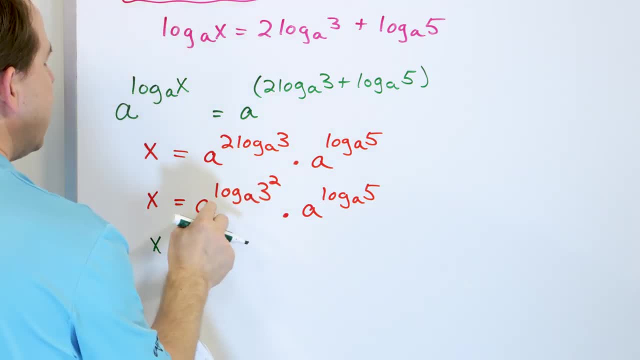 we're very close. We have x on the left. What do we have on the right? The a raised to the power of log base a, the logs in the a completely cancel. All I have is three squared. This cancels, cancels. I have. the number comes and drops down The a and the log base a cancel here. 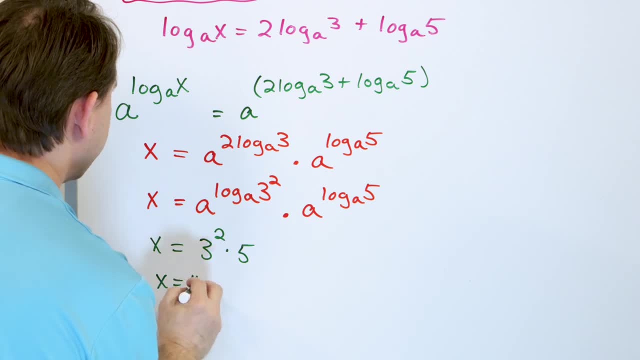 leaving me with five. Now I have nine times five. X is equal to 45.. It's exactly the same answer we got here. Now you might look at this and say, oh, there's more steps. I don't like that, Oh. 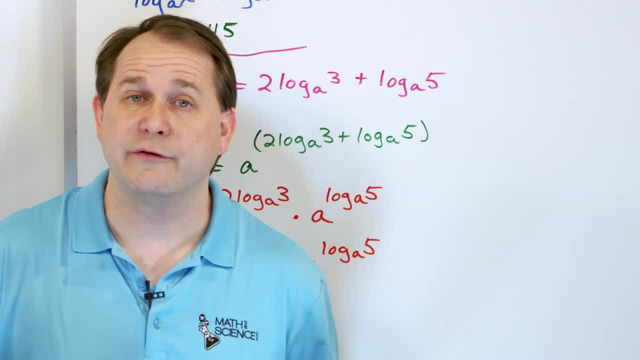 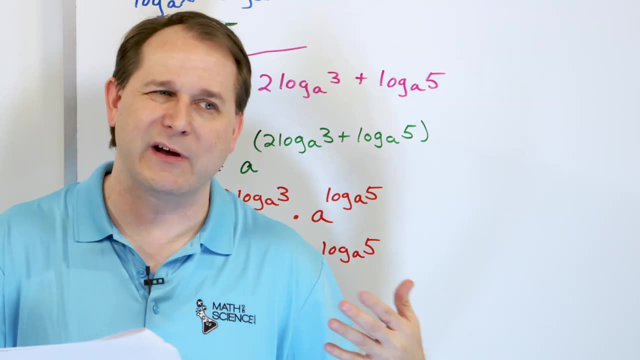 there's fewer steps. I like this. I'm trying to show you both ways, mostly so you understand how it's done, Because later on some equations will be really hard to solve this way, especially in advanced calculus. So I'm trying to teach you the path to get from here to there. 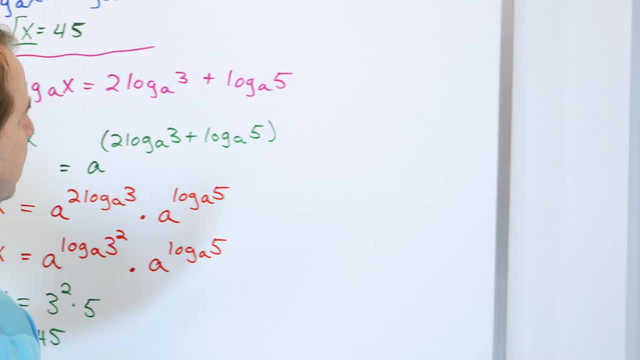 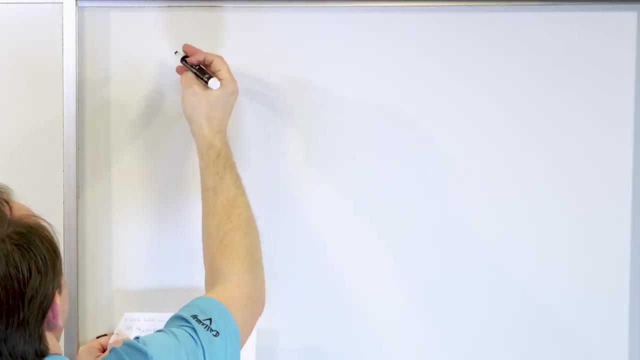 All right, You get the same answer either way, But you have complete freedom on how to proceed. as long as you're following the correct rules, All right. Let's go back to a little more of an easier problem. Let's say we have logarithm base b of x plus three. I don't know what the base is. 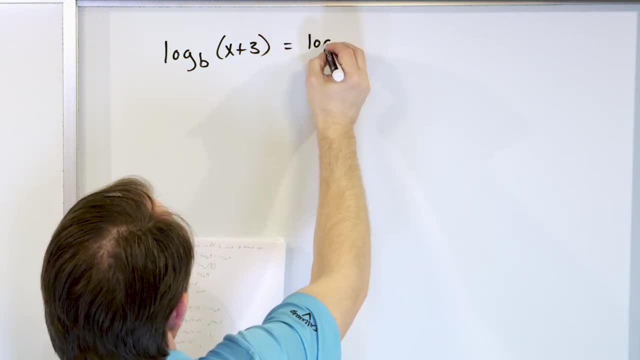 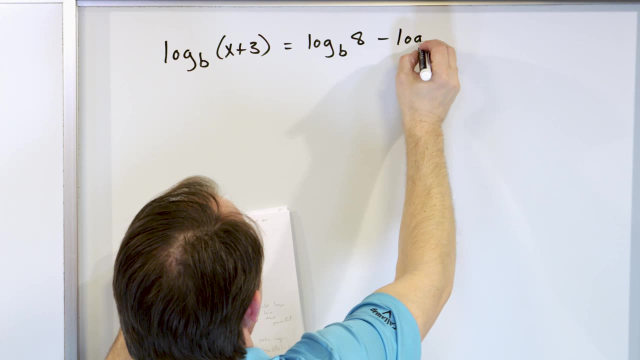 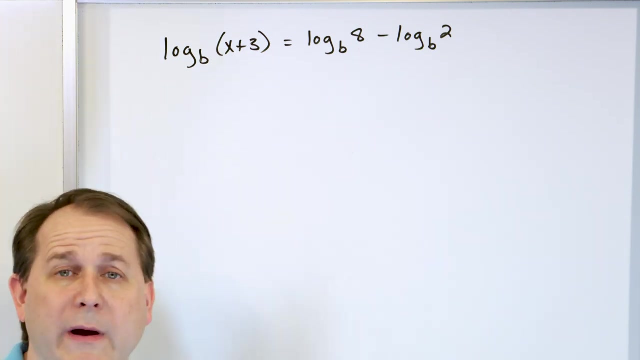 I don't care, It's some. number b equals log base b of the number. let's see if I can erase this of the number eight minus log base b of the number two. All right, So there's lots of different ways to do this. I'm not going to solve every problem. two: 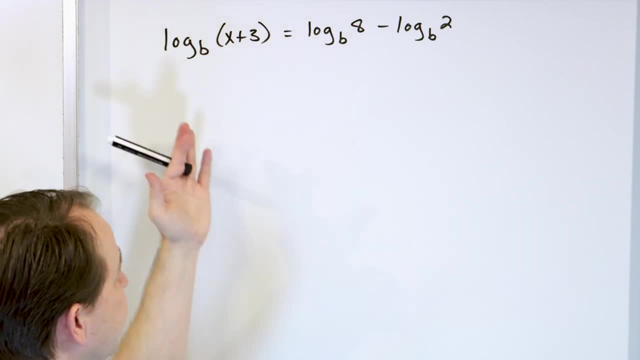 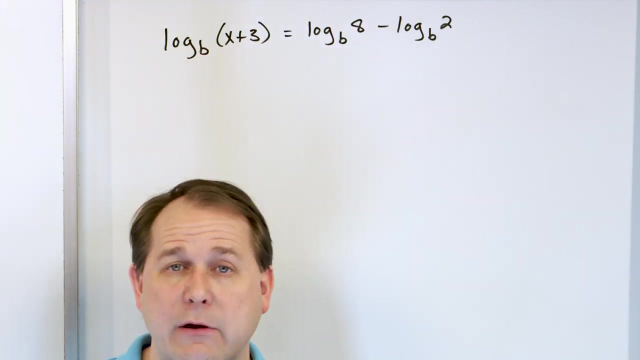 ways right, But you by now know that there's two ways to do it. I can use the laws of logarithms, which is how most textbooks will probably show you, Or I can, because I want this variable x to pop out. I can raise both sides, base b raised to this and then base b raised to that, And I'll 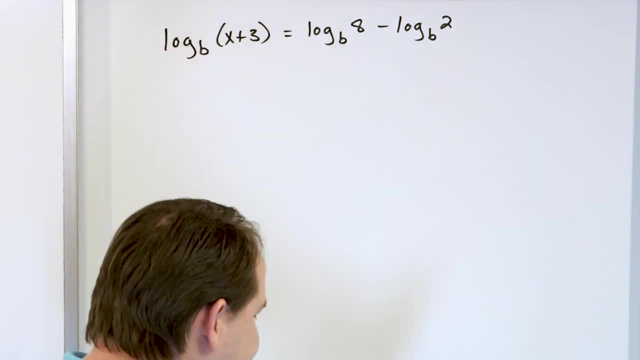 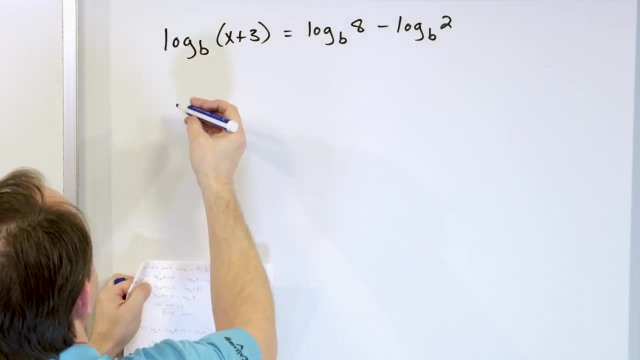 get the same exact answer either way, just like I did in the last problem. So you have to pick a way. There is no correct way. I will do some problems one way and some problems the other way. This way, let's just use the laws of logarithms, Log base b, x plus three On the right-hand side. 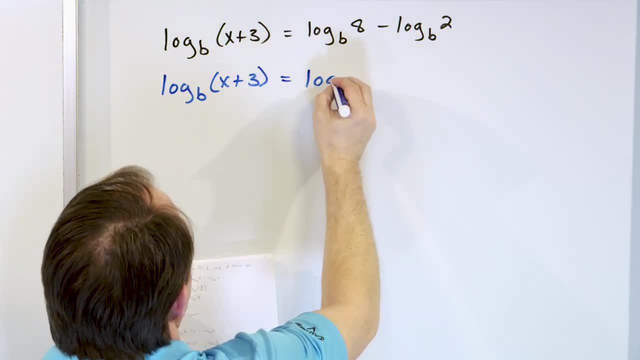 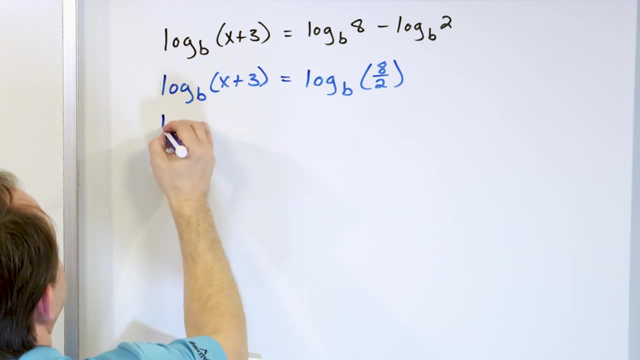 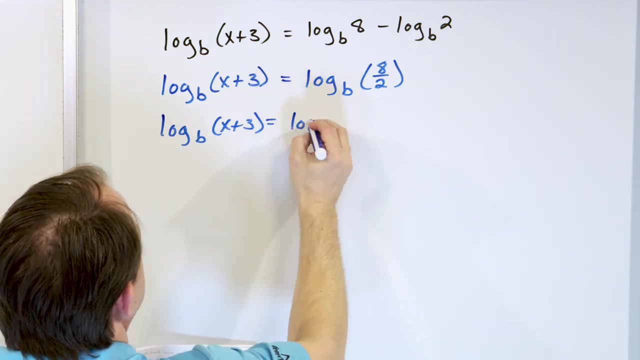 what do we have? A subtraction of logs, So I can write this as log base b of eight over two, because this minus this becomes division eight over two. So what I'll have is log base b: x plus three equals log base b of what? Four. Now you see what you have: Log on the left, log on the. 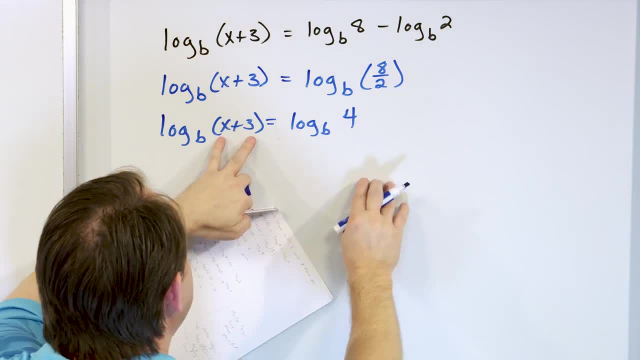 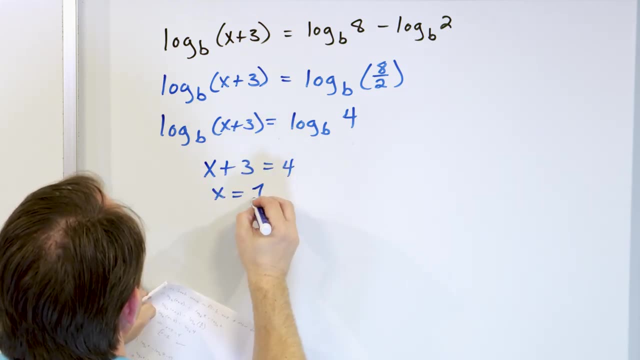 on the right base b, base b, everything's the same. so that means this thing inside of the log has to be equal to four. x plus three is equal to four. so then x. when you subtract the three, you just get a one. this is the final answer. now i'm not going to solve every problem every way, but if you were to, 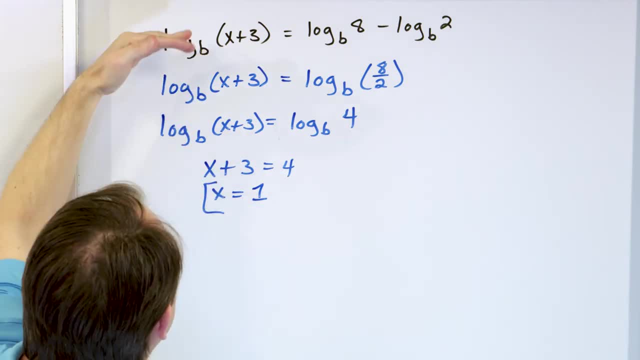 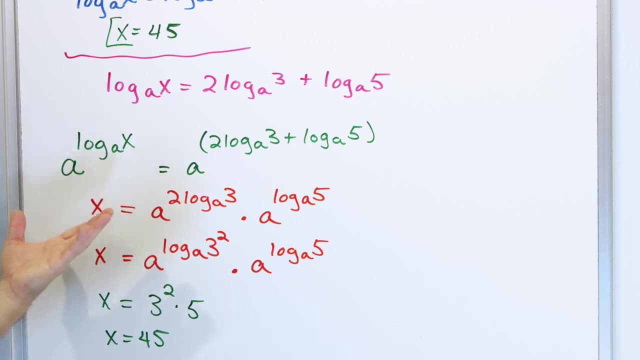 do this the other way. if you would raise the left hand side b to the power of this and the right hand side b to the power of this, it would look really, really similar to what we did here. it's almost the same exact problem. everything would fall out so that you would still get. x is equal. 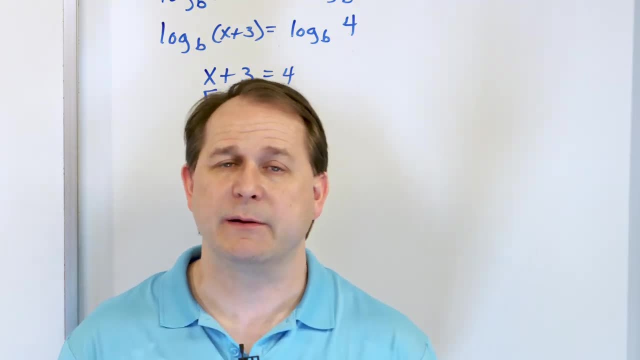 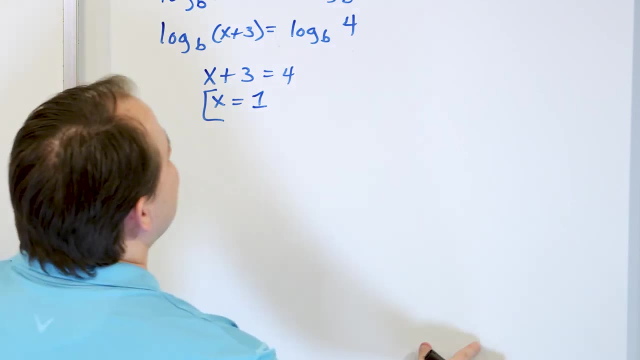 to one. i i'm just, from now on, i'm just going to pick a path. i'm not going to particularly choose one specific way to do things. okay, um, let me slide to the next board to do the next problem, because it's a little longer, and then our last problem is actually going to be fairly short. 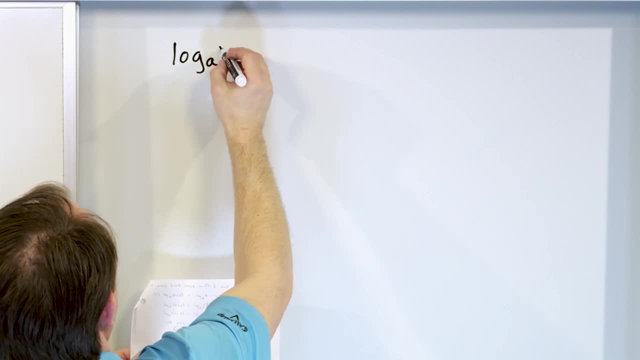 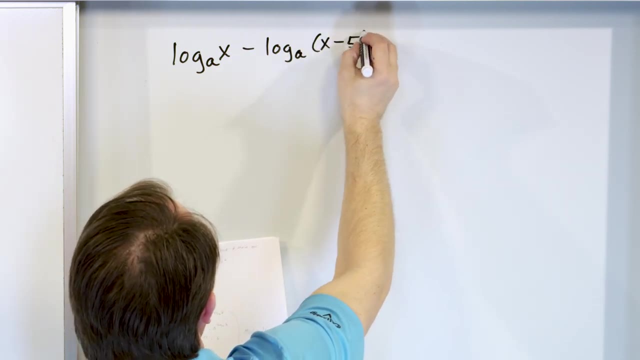 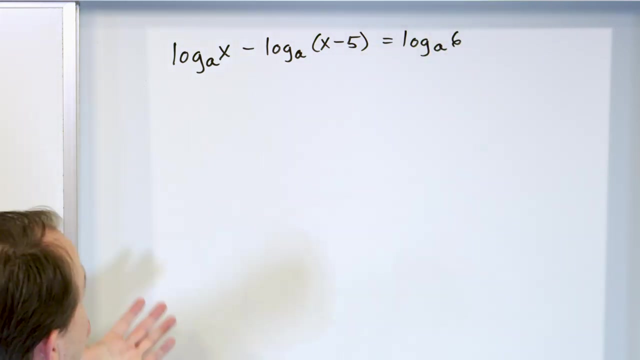 what if we have log base a of the variable x minus? log base a a x minus 5 is equal to log base a of the number 6.. Again, I can do what I want. I can use the laws of logarithms. I have subtraction of two logarithms. I could do that. It would probably. 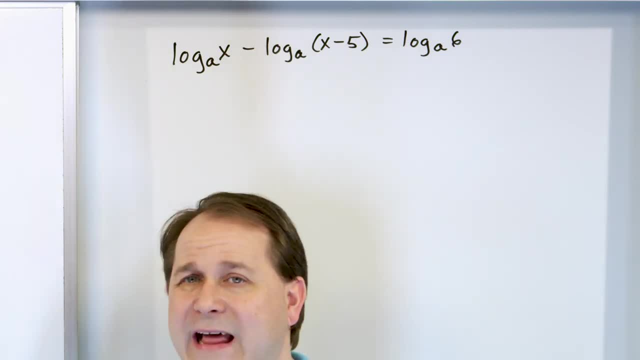 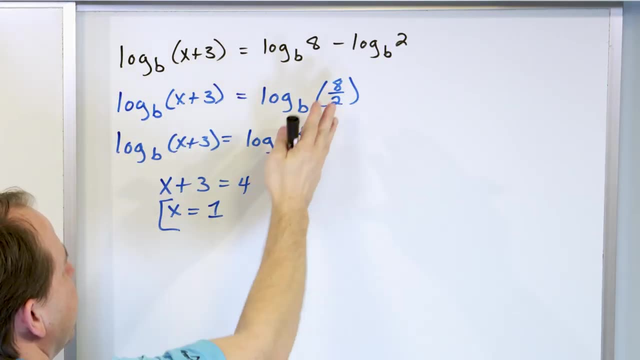 be a shorter answer, just like I did in the last one, But I really want you to understand both ways of doing it. So, instead of doing it like this, where we use the laws of logarithms- it'll probably be pretty short. to be honest with you, Let's do it the slightly longer way, because I 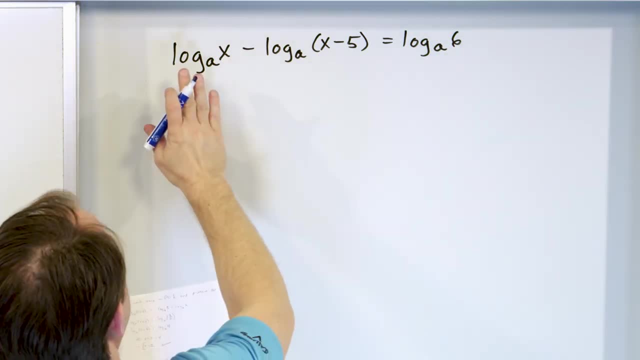 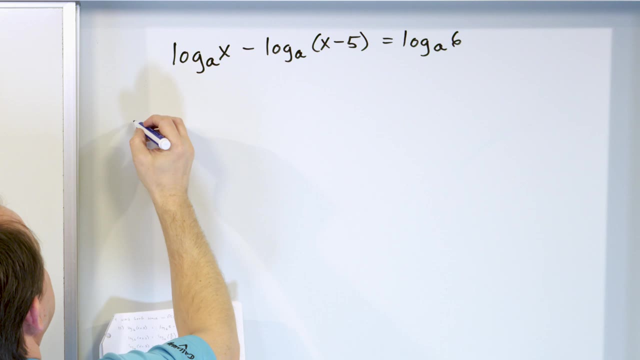 want to show you that both ways work. So here I have log base a, log base a, log base a. So what I want to do is I want to kill all those logarithms. So on the left-hand side, I'll raise it and put. 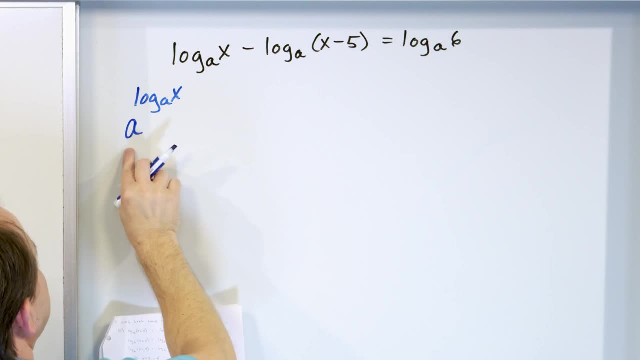 all of this stuff in the exponent of a base: a. This whole thing on the left-hand side, a x minus 5.. This entire thing is in the exponent of a. Over here, a log base: a 6. All right, But again I have a subtraction in the exponent. I have subtraction So I can write this as log. 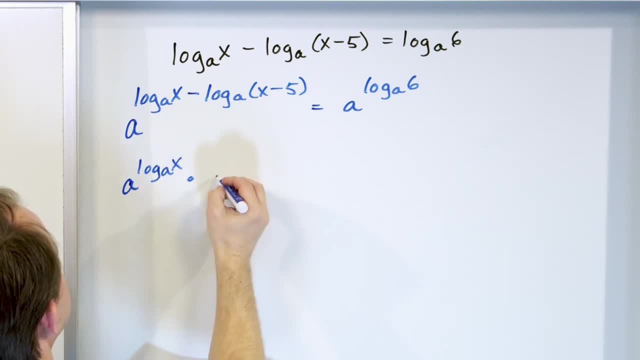 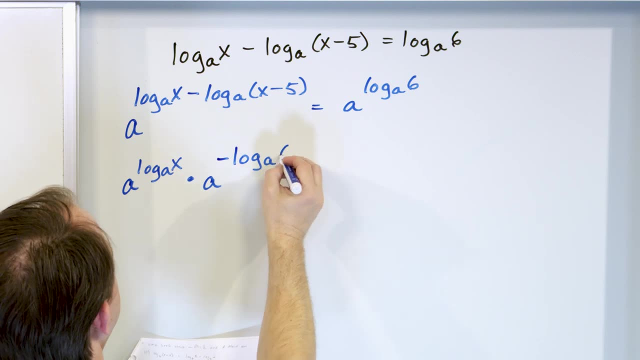 in the exponent a of x multiplied by a to the. how do I want to do this negative log a base a: x minus 5. And on the right-hand side the a is going to kind of cancel with the log a. 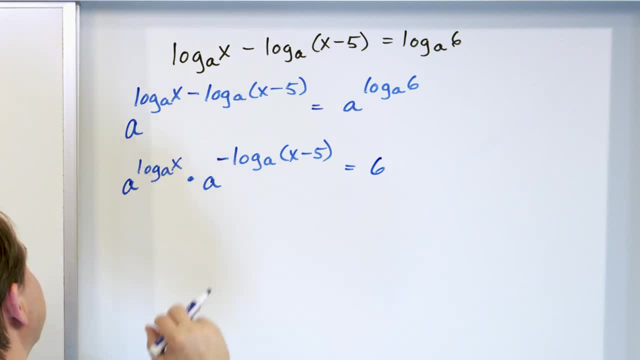 because they're inverses of one another. I'm just going to have a 6.. Now make sure you really understand the left-hand side. All I'm saying is that I have the same base here, so I can add these exponents. 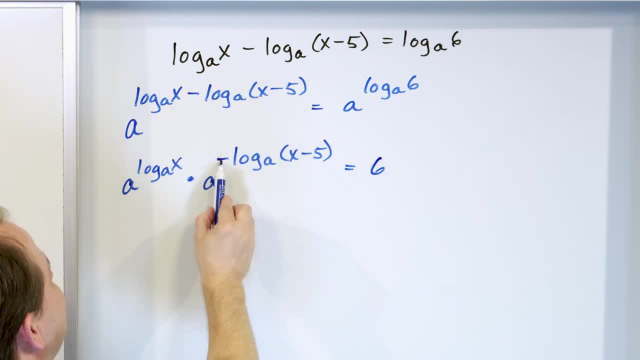 If I add this to this in the exponent, I'm going to get exactly what I had before. That's why I had to have the negative sign there, because ultimately they're subtracted, So I can work in kind of the exponential kind of realm if I want to. Now, what do I have? This log base a cancels. 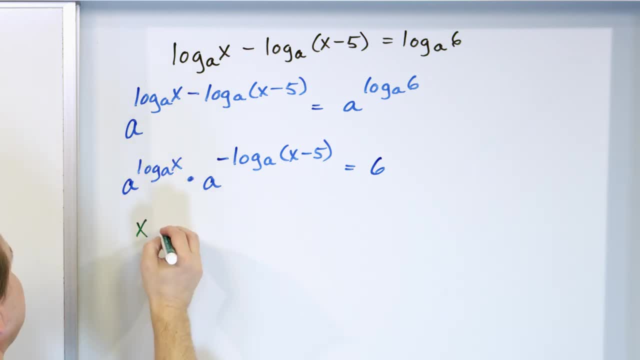 with this exponential, with base a. so I just have the x popping out from the top. This a cancels with this. However, there's one little gotcha here. You have a negative sign in front Before you can do the cancellation. this is like a negative 1 out here. So what I want you to do is: 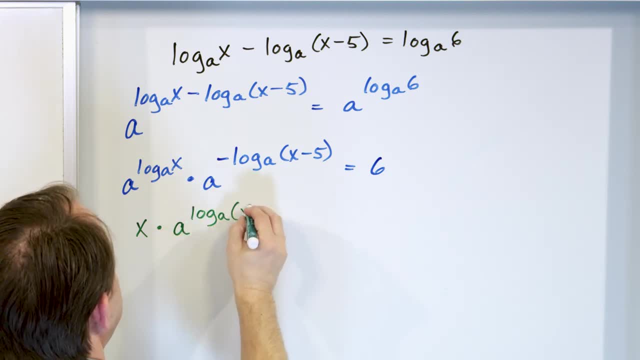 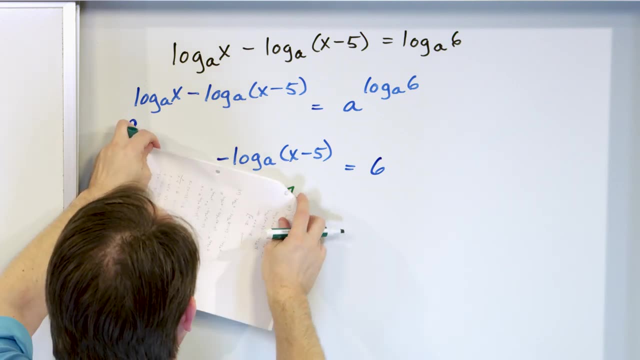 say, log base a x minus 5 to the negative 1 power. This is like a negative 1 times this. So forget about everything else here. If you just had this- this negative 1, you can float it in and put it as: 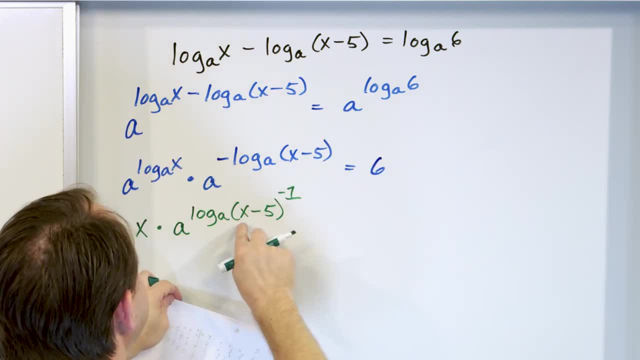 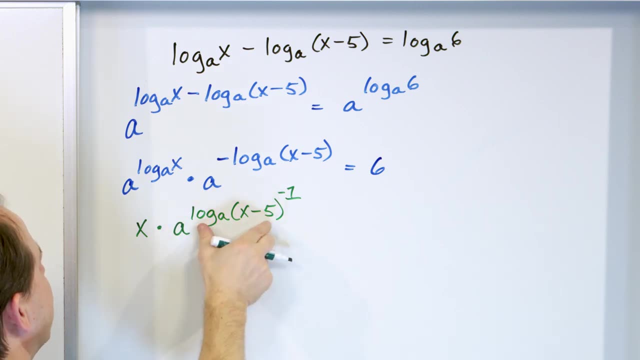 a power. Log base: a x minus 5 to the negative 1. Log base: a x minus 5 to the negative 1. I want to get rid of it here and bring it here. so now I have a very clean cancellation, a cancelling with. 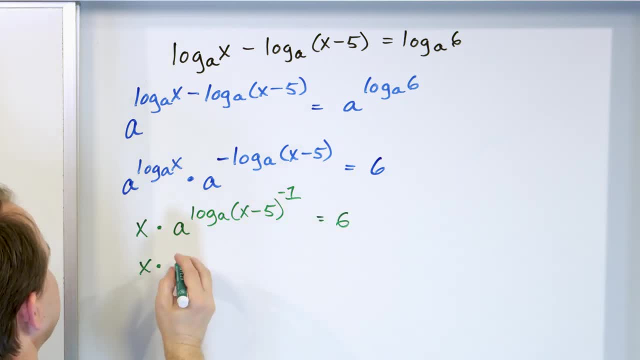 log This is equal to 6.. So I'm going to have x multiplied by x minus 5 to the negative 1 power. The a as a base cancels with log a. so all I have left is x minus 5 to the negative 1.. Let me just 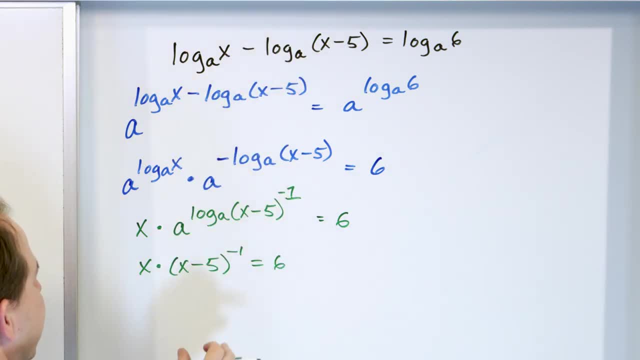 double check myself, And so now I'm home free. I've got rid of all the logarithms. Now it's just a basic algebra problem. Let's bring this to the bottom: x over x minus 5 to the first power. I 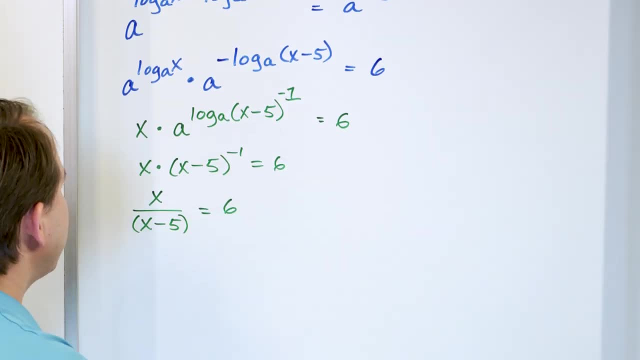 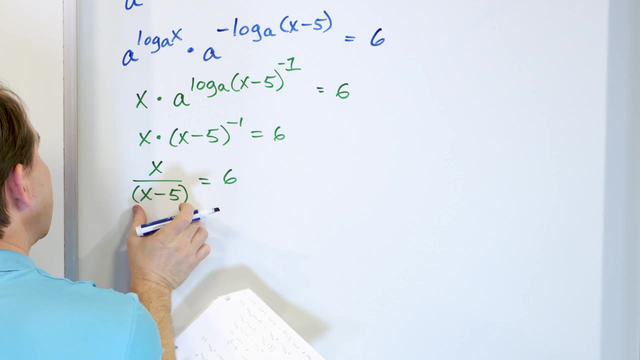 can drop the parentheses or leave them there, whatever you want, 6.. So I have to solve for x. So I'm going to multiply the left and the right-hand side by the denominator x minus 5.. On the left I'm going to be left with x. On the right it'll be 6 times x minus 5.. I 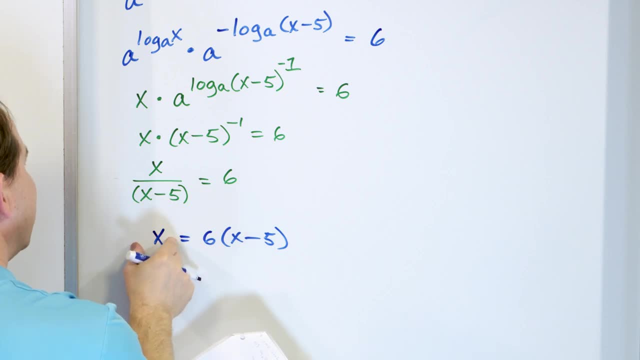 multiply the left by x minus 5. It cancels. That's what I'm left with. On the right, I multiply by the same thing. Here's what I have. So I have now 6x minus 30 when I distribute this in And then 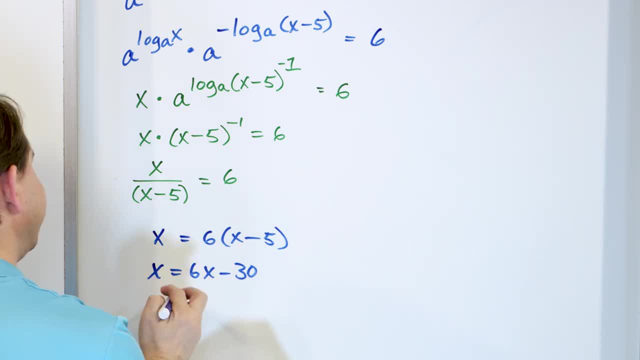 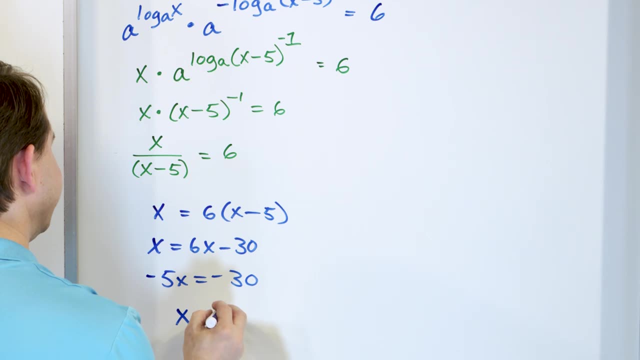 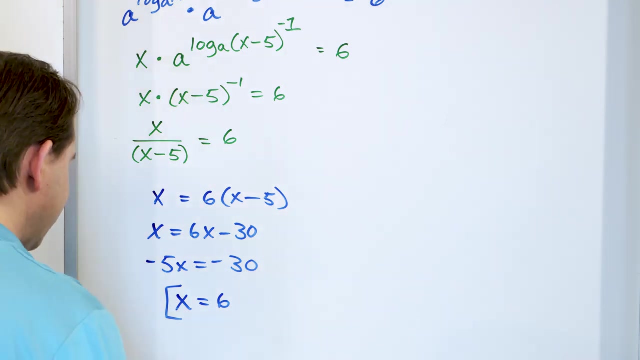 I'm going to move the 6 over here by subtraction, So 1 minus 6 is negative 5x, And then I'm going to divide by negative 5. I'm going to get a positive 6.. x is equal to positive 6. That's correct. And again, there's always more than one way to do. 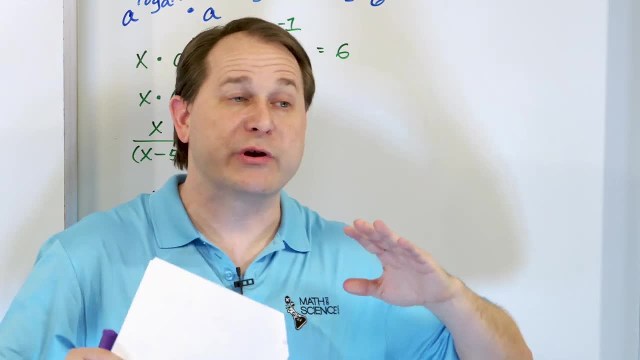 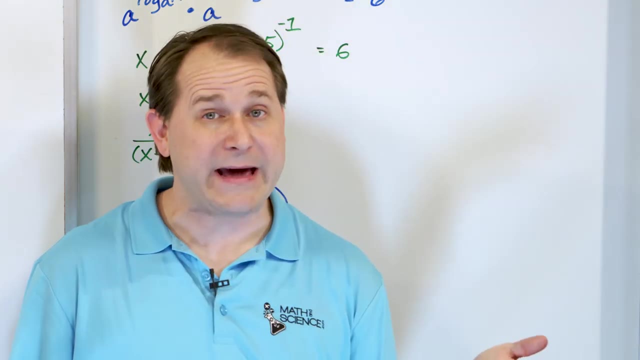 the problem. But in this case I wanted to really show you that if you have logarithms running around your equations, just kill them with exponentials: Raise the left to an exponential, the right to an exponential- same base- and all of those logs will get eliminated. Now, just for. 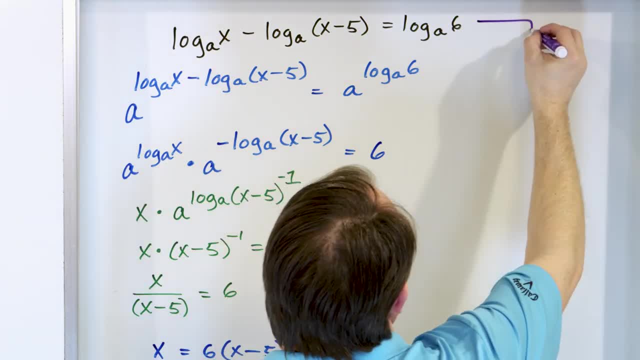 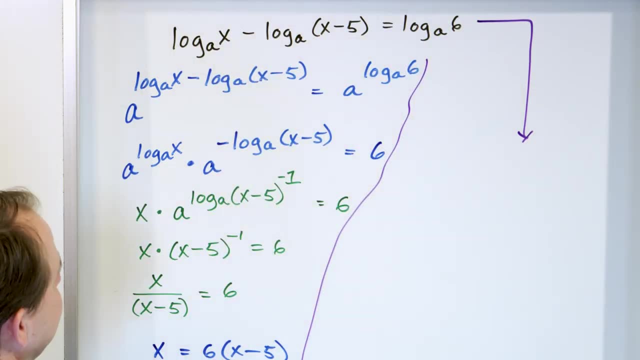 giggles. I want to make sure you understand that there's obviously an equivalent way of doing this here. So let's go down here and I'm going to show you. We're going to start with the black line. How would we do it? just using the laws of logarithms. 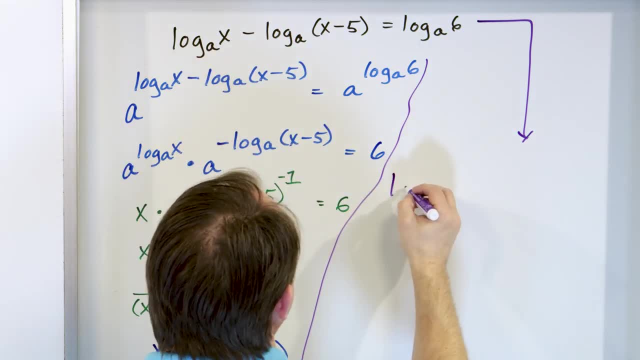 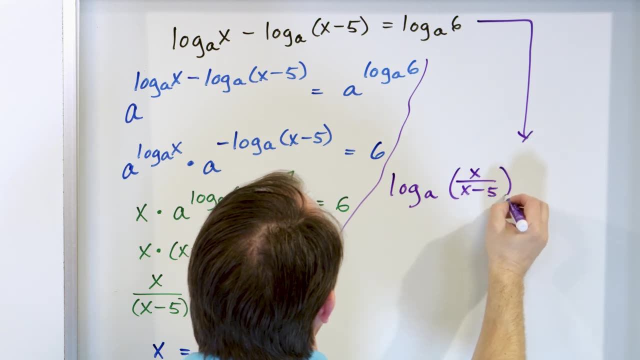 I have a logarithm minus a logarithm, So I can write this as a division: Log base a of this, divided by this x over x minus 5, equals this Log base a, 6. So you see, just with a simple line. 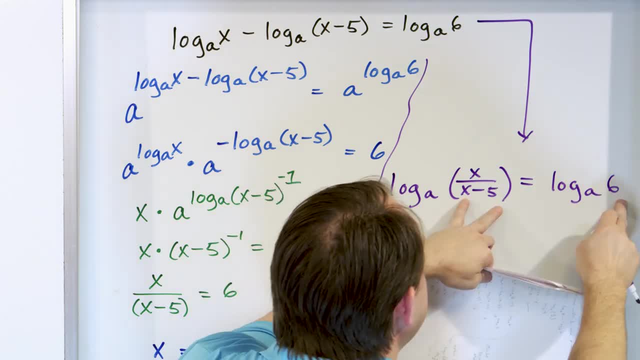 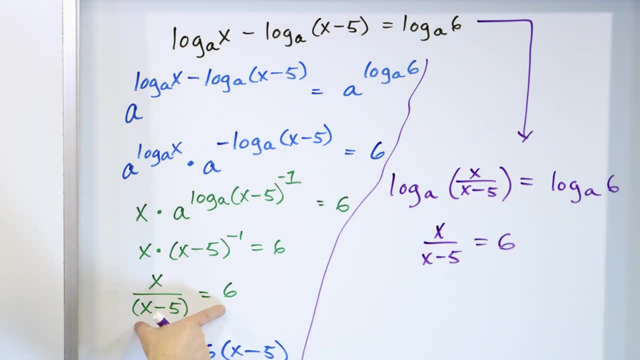 I now have base a logarithm. base a logarithm And the thing I'm taking the logarithm of. they have to be equal. x over x minus 5 is equal to 6.. That's exactly where I arrived right here. x over x minus 5 is 6.. So from here, the solution's the 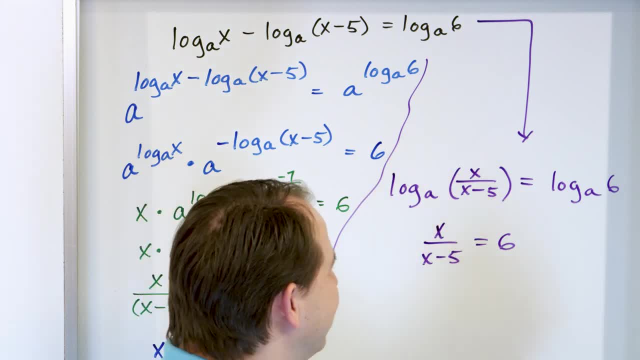 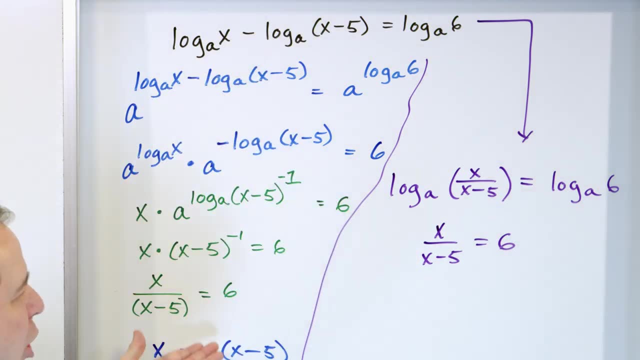 same, You would get the same thing. I agree with you that this is fewer steps. This is typically what you would see in most textbooks, especially at the introductory level. But I really want you to understand how logarithms and exponentials can annihilate each other, because when you get 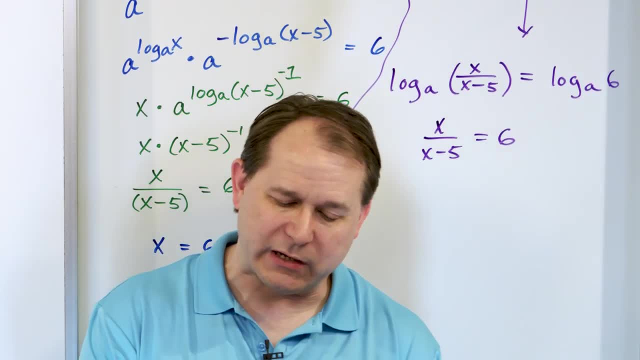 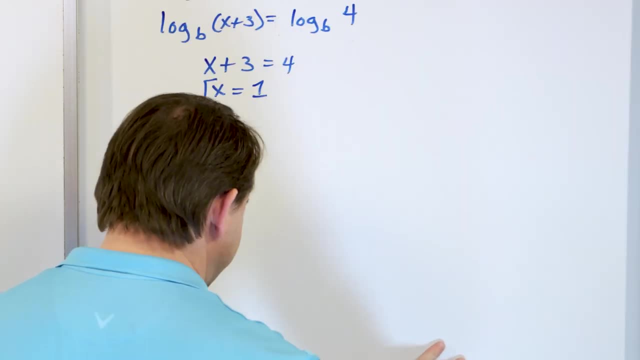 farther along in math, it becomes incredibly useful, And so I want to make sure you understand that. All right, we have one more problem. It's actually not a very long problem, So I'm going to slide back here and do it underneath. 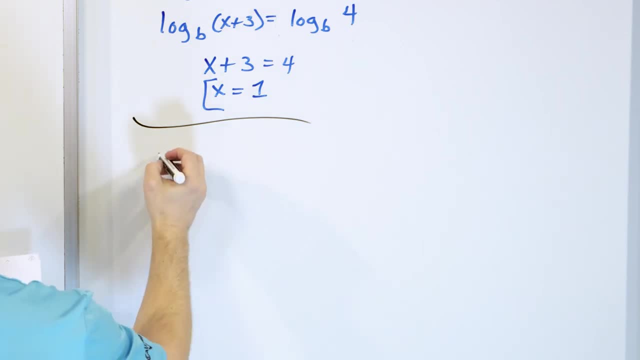 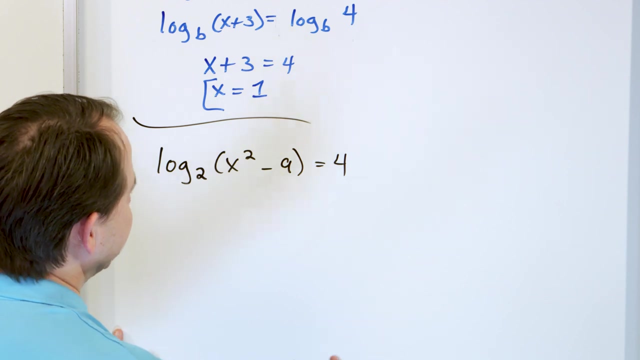 But it's a good problem. What if I have logarithm base 2 x squared minus 9 is equal to 4?. Now I just got through telling you I can kill the logarithm with an exponential. I can raise both sides to an exponential with a base 2.. I can do that. But instead of doing that, let's just use 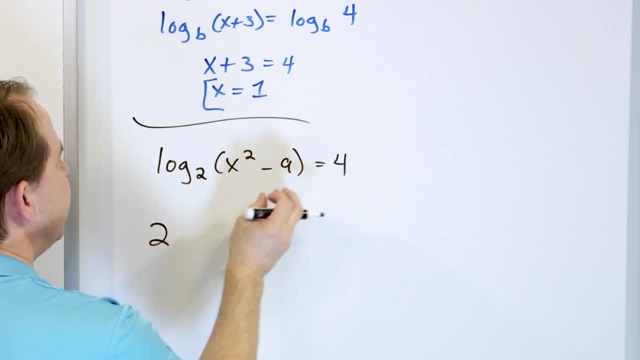 the definition of a logarithm, just for variety: 2 to the power of 4 is equal to what this is inside the logarithm x squared minus 9.. Now the logarithm is again gone. 2 to the power of 4 is 16, x squared minus 9.. I'll move the 9 over. 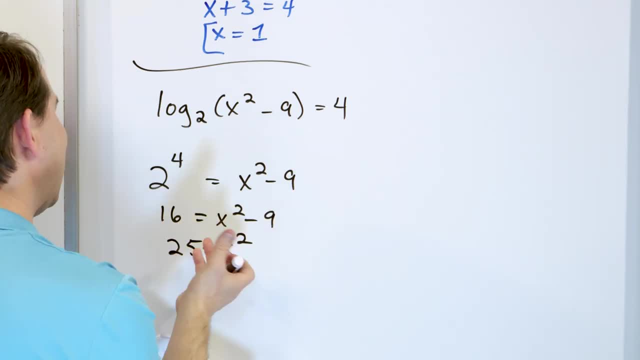 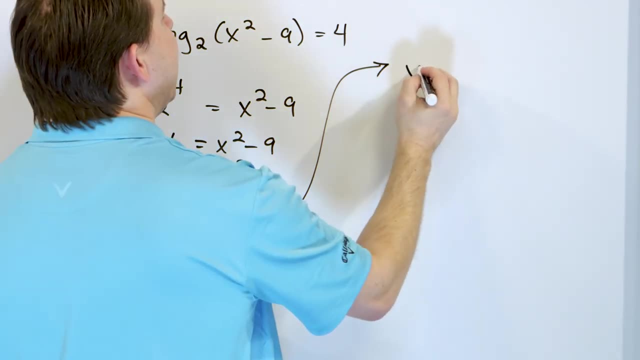 by addition, I'll have 25 equals x squared. I never like having it like this, So let's flip it around 25. And then we'll go over here. I think you can see what the answer is going to be. x is. 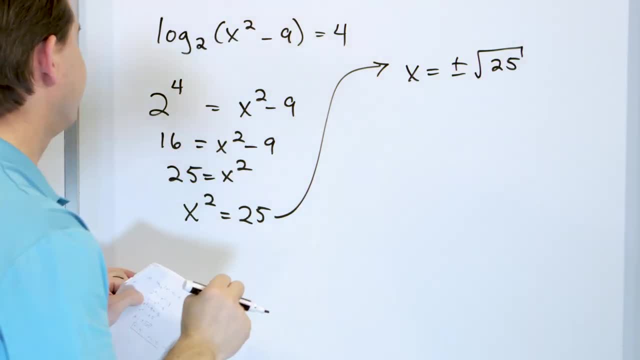 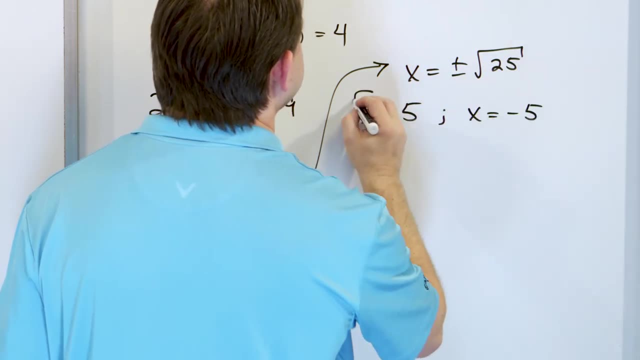 going to be plus or minus the square root of 25.. But as I take the square root of both sides, so x can be 5, x can be negative 5.. So that's the original answer: x is 5, x is negative 5.. You have two answers. You might say: 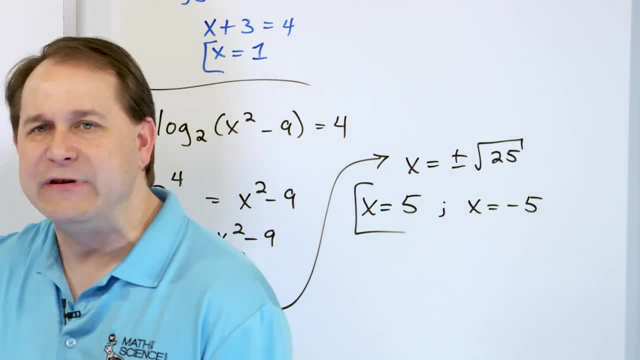 whoa, whoa, whoa, whoa, whoa. You just told me that I cannot have negative numbers feeding into a logarithm. You just told me I cannot have negative numbers going into a logarithm, So why do I have? 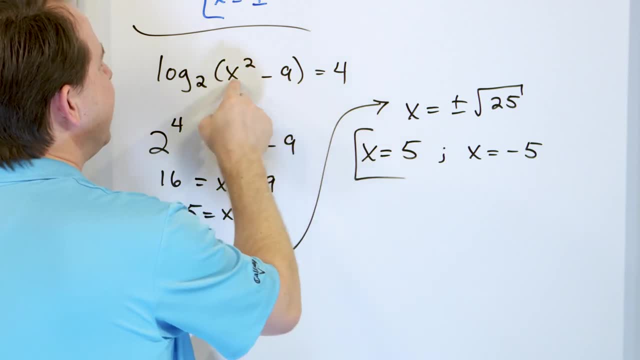 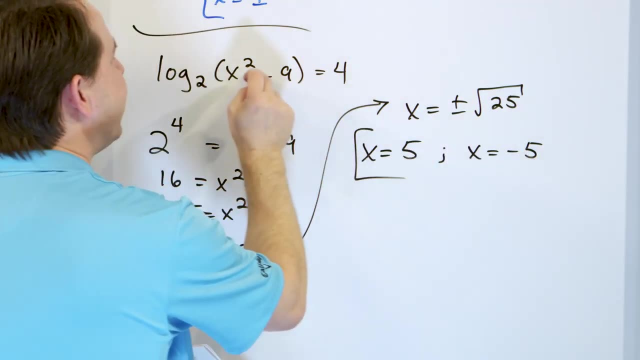 two answers here. Well, here's why: If I put 5 in here, it's squared, That's going to be 25 minus 9.. That is what I'm taking, the logarithm of a positive number. If I put negative 5 in here, I